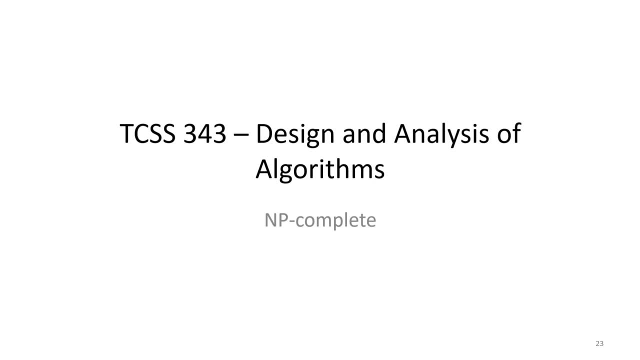 All right, welcome This video. I want to finish talking about NP complete problems. We've sort of prepared ourselves by talking about decision problems- the complexity class P and the complexity class NP- and I sort of want to finish filling in the picture now by defining NP complete. 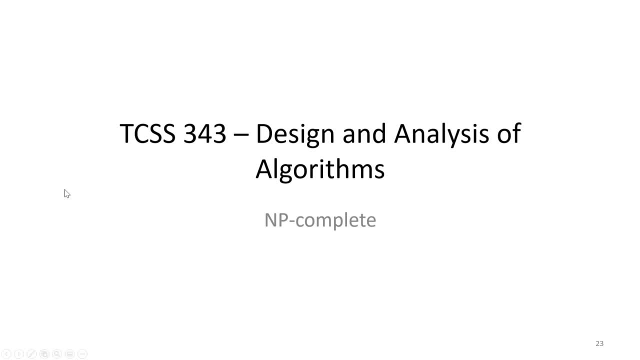 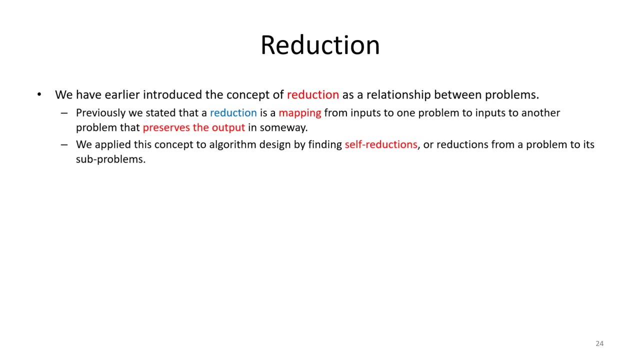 problems. So there's a few more steps we need to take before we get there. so let's continue Now. critical or core to the idea of NP completeness is going to be this idea of a reduction, and so far, if you've been following along, we've been using self-reductions to come up with 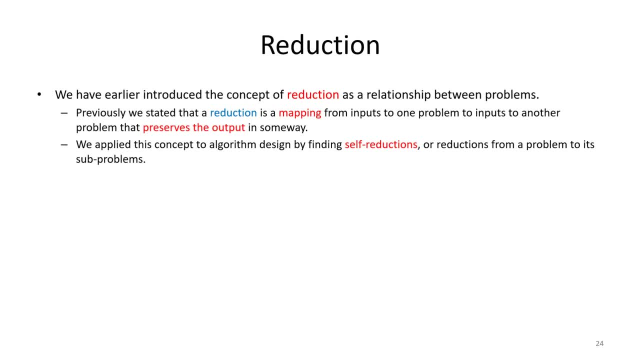 algorithms, and here I've been using this term self-reduction sort of loosely, without really defining what I mean by reduction. Well, reduction is a way to relate two problems, usually, but a self-reduction then is one where a problem is related to itself, and that's sort of what we've been focusing on so far. 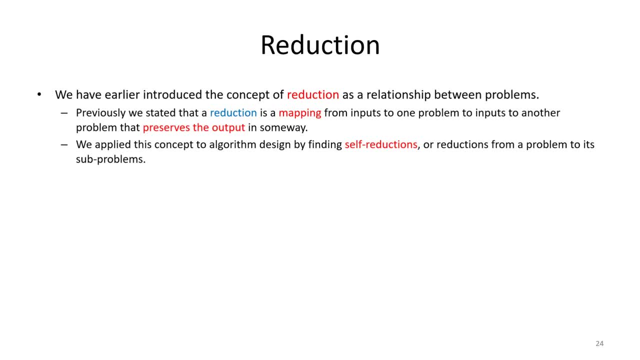 but now I want to shift gears and look at reductions, not just from a problem to itself to its sub-problems, but instead a reduction from a problem to another problem, usually a closely related problem, and I've sort of been highlighting this in the earlier videos, Whenever we'd encounter. 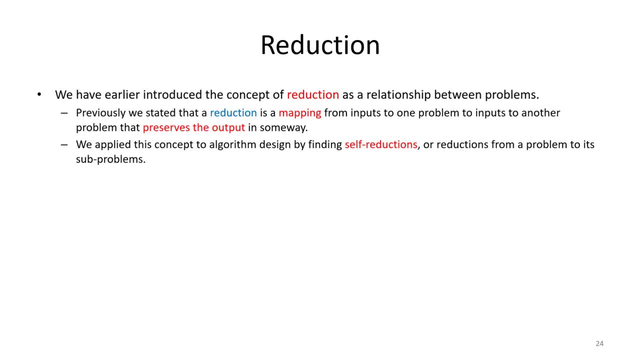 a couple problems, I'd say, hey, these are really closely related problems. Is there a way we can formalize that now and actually prove that? And so I'm going to start by saying: well, how can we prove that they are closely related, somehow give evidence that this relationship is strong? 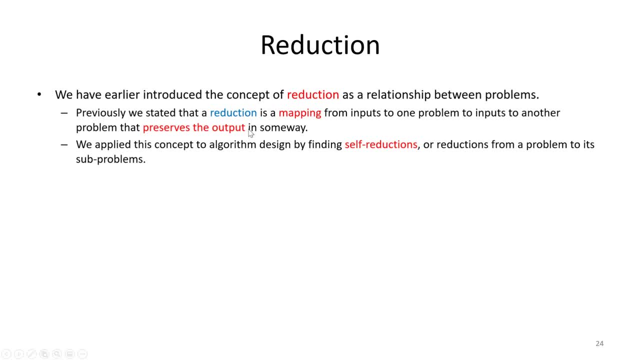 And so to do that, we're going to rely on this idea of a reduction. The reduction, loosely informally first, a reduction is going to be any relationship between any mapping, between the problems, where we're now mapping specifically inputs, that- and here's the key part- that preserves the output in some way. 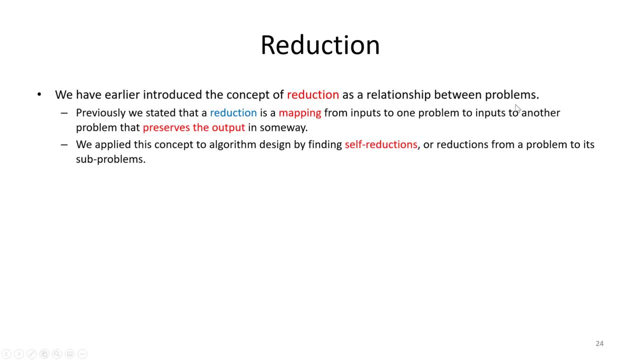 Here I'm being a bit vague. So we've got our two problems. maybe call them problem A and problem B. So we've now got this mapping. that's a function that's going to take the inputs of problem A and turn them into inputs of problem B and preserve the output in some way. What do I mean by that way? 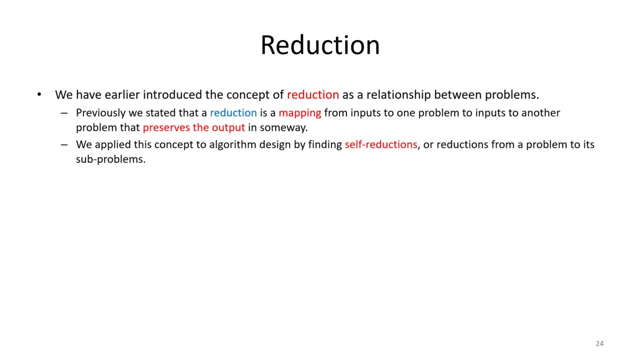 Well, one way you could preserve the output is if the output was exactly the same when after you do the change. that would be perfect presumption: Preservation of the output. But we can imagine some other way, basically some way that we could extract or recover the appropriate output afterwards, And I'm going to flesh that out a little bit. 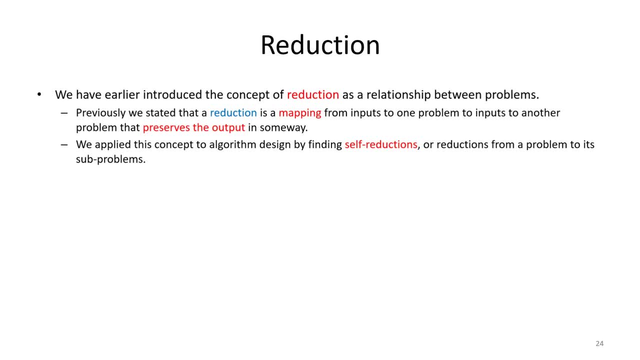 So that's sort of an informal idea of what a reduction is, And there are a number of different kinds of reduction. One is the self-reductions that we've been looking at already, But another kind is the kind that we're going to focus on now, and it's going to be called a Cook reduction, or, more commonly, a. 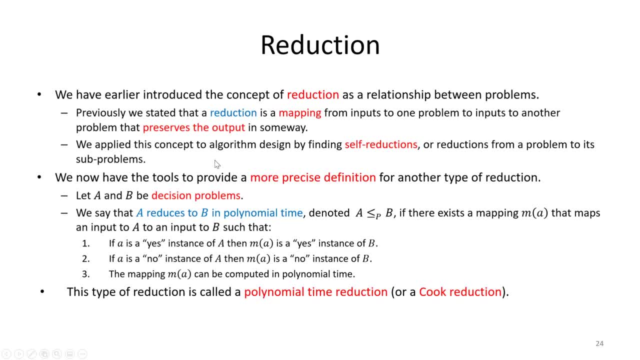 polynomial reduction. It's a real-time reduction And here's where I'm just going to lay it out, with its formal definition and some of the parts we've sort of already been hinting at already. So first of all we've got two problems. I want to again. 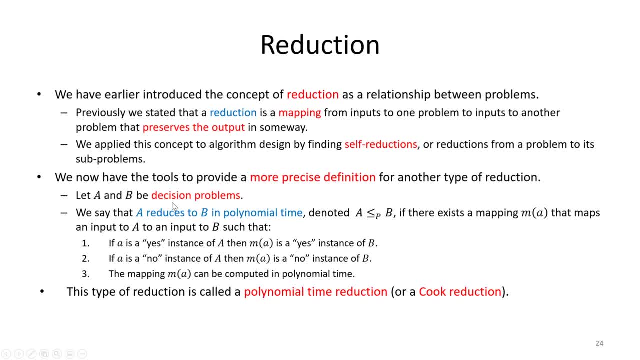 be a little bit more precise and say what kind of problems? Well, let's make them decision problems. This is going to make it easier for us to handle the preserves, the output component, because decision problems always have the same output: Yes, no right. So hopefully this is going to set things up to be a little bit easier for us. Now let's take a look at our 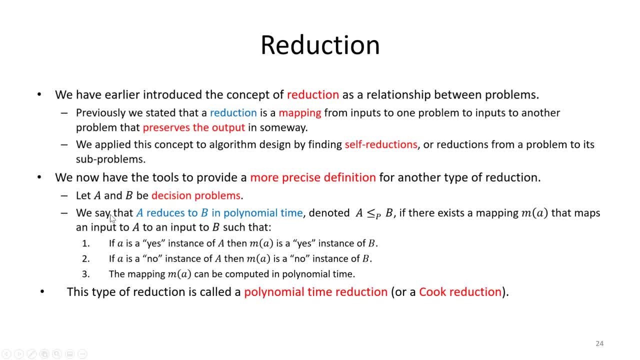 definition. Everything down here is the definition. It's a little bit more, but let's take a look. So first of all, we're just setting up how we're going to use the term. We're going to say A reduces to B, and then often we'll say in: 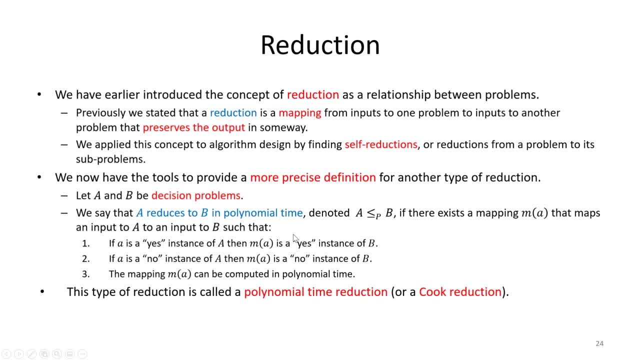 polynomial time, unless it's already understood. And then here's how we symbolize that. Here's how we denote that with symbols. We're going to say A is less than or equal to B. The less than or equal to symbol here is being borrowed, And we'll see in a moment why we've chosen that one, But we're going to use that as sort of our 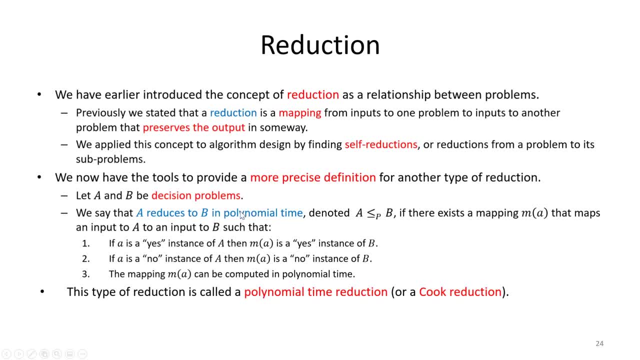 symbol for reduction And then the P. here is the polynomial time part. OK, there are other types of reductions that we might encounter, And so, to signify which type of reduction we're using, we're going to use P for polynomial time. OK, so this is just setting up how we're going to use it. This is what we're defining. So what does it mean when we use this? 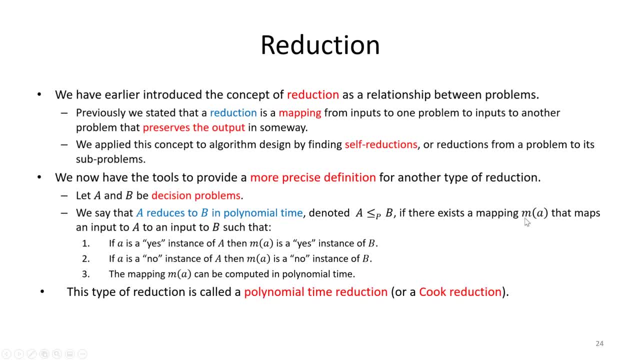 symbology. Well, here it means that there's going to exist some map, OK, and there's a function on map where A is what its argument, whatever it's taking, and it's going to map an input to A to an input to B. So here's that mapping we were talking. 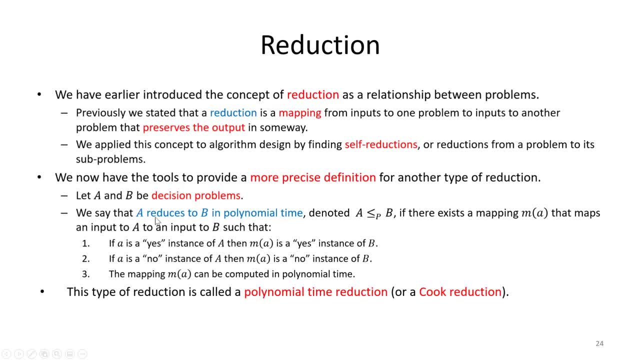 about before, And it's going to change the inputs to problem A into inputs to problem B. Now here we need to think a little bit abstractly. Problem A and problem B- we don't really know what they are. Remember, fundamentally we said that their inputs could be interpreted as binary strings, So this: 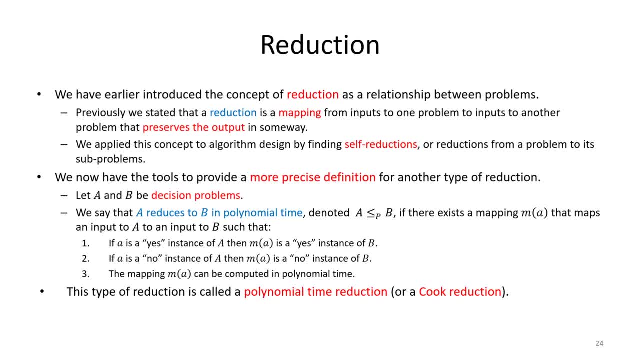 mapping fundamentally is going to be binary into binary, But not so fundamentally. thinking about the problems themselves, our inputs to any given problem depends on the problem. We might have a graph in one case, then we might have a set of integers in another, or we might have a set of points, or we might have a. 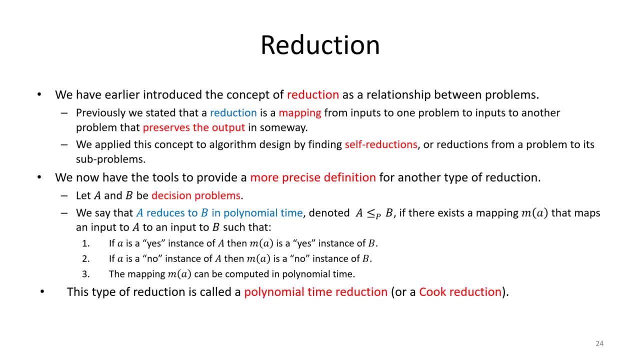 geometric figure. There's so many different possible things that we might be taking as our input that we need to be careful here, And we need to recognize that coming up with this mapping is going to require a great deal of cleverness on our part, And some mappings are going to be. 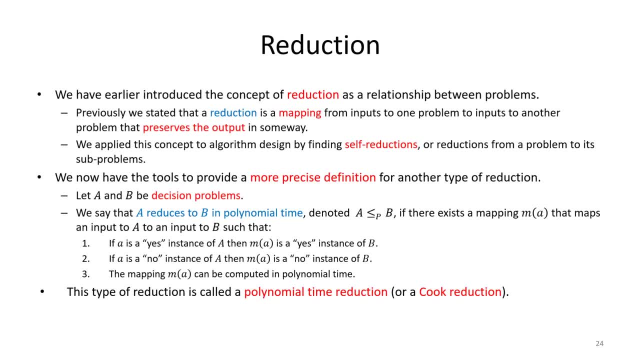 easier to come up with than others, than others- and I might highlight this a little bit more- as we encounter them Now. so coming up with a mapping that maps from one input to another, as I mentioned, might already require some cleverness, especially if we're changing from one type to another. 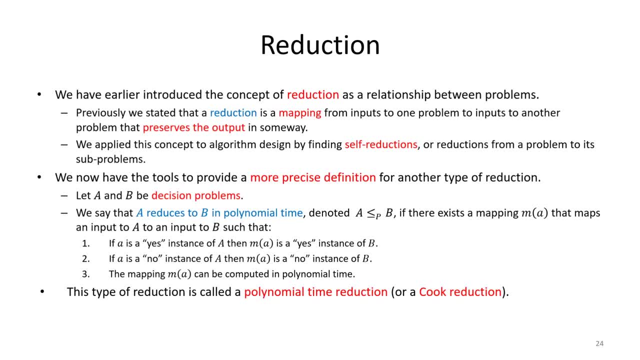 But sometimes it won't be that hard if we have, say, graphs turning into graphs. But still we can't just accept any old mapping that just takes any input and maps it to any input. We want to preserve the output And so the first two criteria that we have here on our mapping is basically saying that 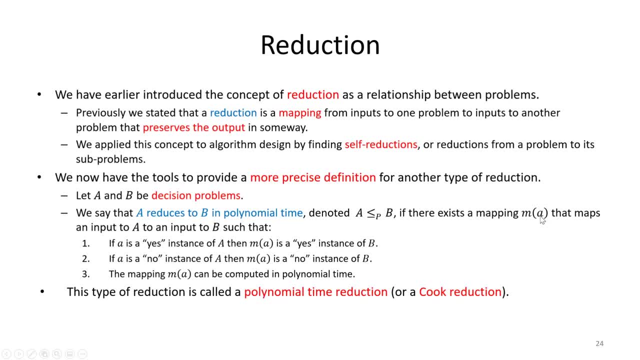 for a decision problem. It's saying that if A- the input to A was yes- was something we should say yes to, we'll call that a yes instance of problem A. then whatever we map it to, which we know is going, 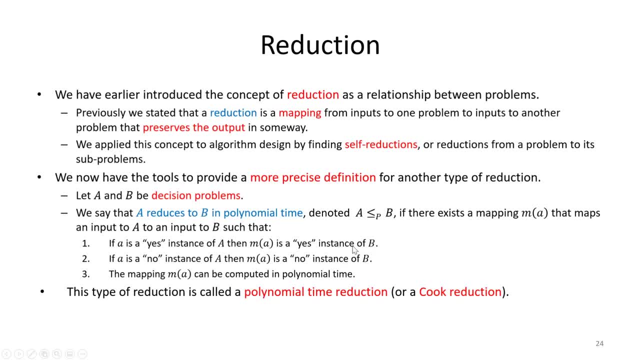 to be an input to problem B should still be a yes instance. So yeses get mapped And then the parallel statement for noes. If A used to be a no instance, then it should be mapped to a no, And this is the preserving the output bit. 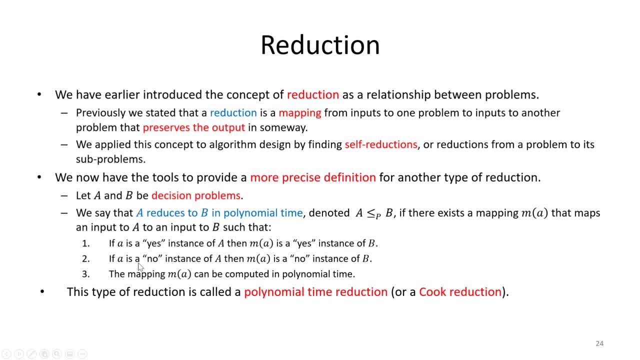 And in fact if we ignore condition three here, we can erase the P there and we might get ourselves a different kind of reduction. The polynomial time criteria here, saying that M is polynomial time computable, is what the P stands for. 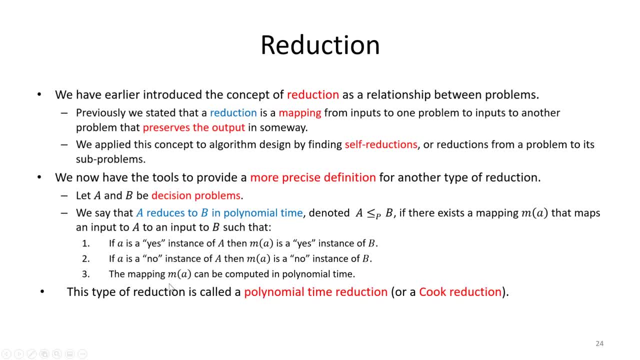 Other types of reduction will probably still want us to preserve the output, but they might have a different criteria on the mapping. For instance, a Turing reduction which is sort of this is a more specific or a more restrictive reduction than a Turing reduction. 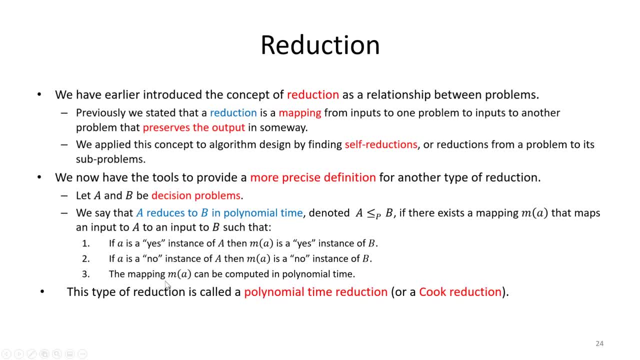 It replaces condition three with just the mapping M A can be computed, period. It doesn't tell you how much time it's going to take to do it, It just can be computed, Even if that takes a really long time. If you do that, then you're going to get a slightly different kind of reduction useful. 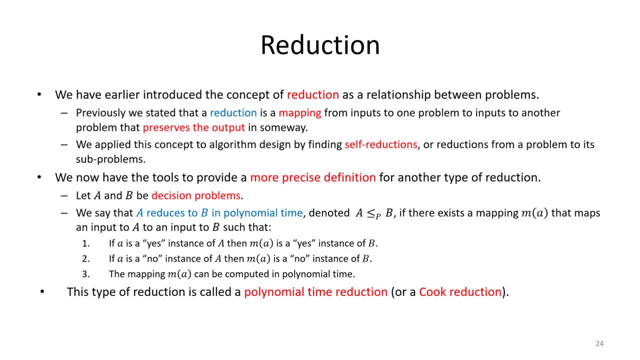 in computability theory We're doing complexity theory. So this Cook reduction, this polynomial time reduction, here is what's useful for us in complexity theory. So again, that's just meant to highlight differences between reductions, But again, this is the reduction we are going to use. 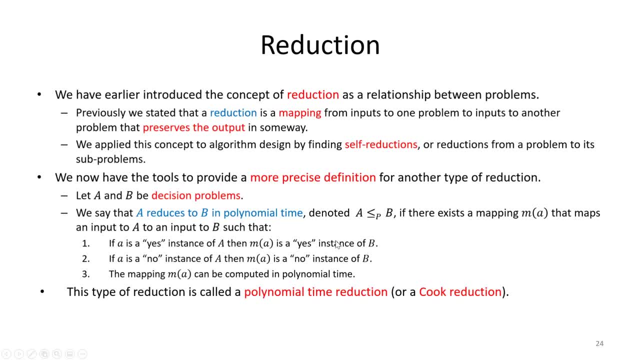 It's important that we confirm that our mapping afterwards, First, that it preserves our output- yes to yeses and noes to noes, But then, if we've got that, we want to make sure that we haven't done anything that might. 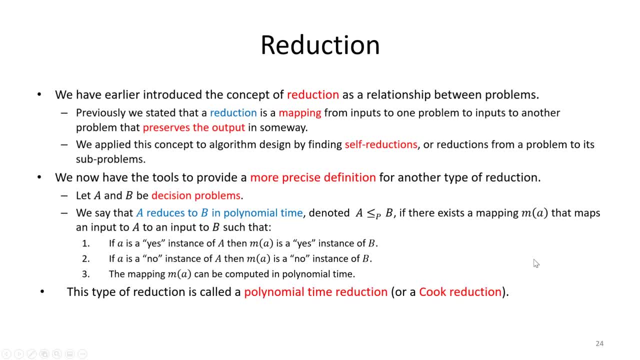 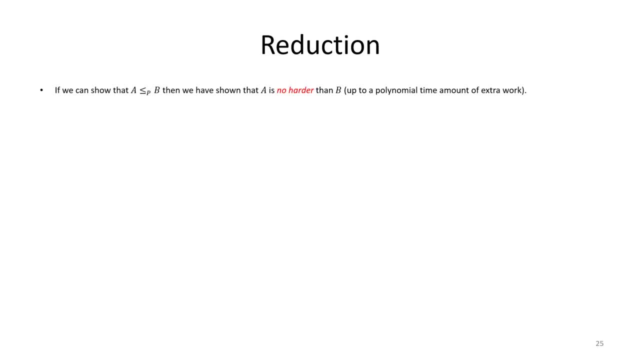 take more than a polynomial time. Okay, let's see how this idea of a reduction is going to help us talk more about problems in NP. Now the first thing is: how can we interpret what this reduction is telling us? That definition is sort of involved. 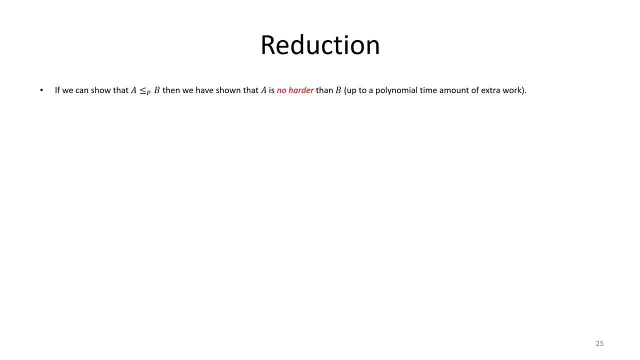 It doesn't really say too much. I want us to build up our intuition that the less than or equal to there the reason we've chosen that is because what we're really comparing here is the complexity of our two problems, and the less than or equal to is really trying to express that, that the complexity. 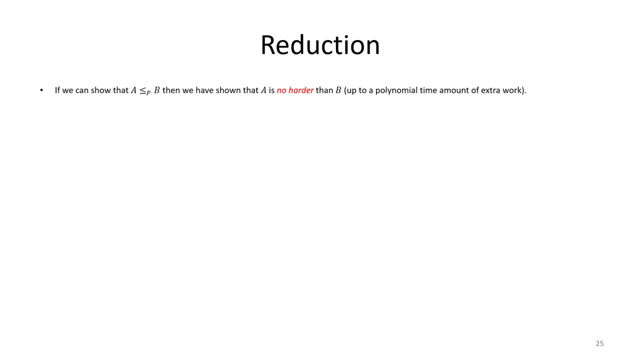 of A is less than or equal to the complexity of B, And so another way of saying that is that problem A is no harder than problem B. Now you can take my word for it, but I want to sort of justify it for you here. 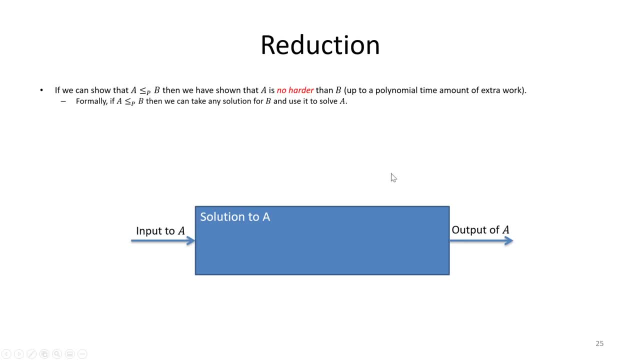 And to do that I'm going to use sort of a picture, a diagram here, where what I'm going to do here is I'm going to use this sort of box diagram where I've got this box, I've got it labeled. this is a solution to problem A, where into the box comes inputs and out. 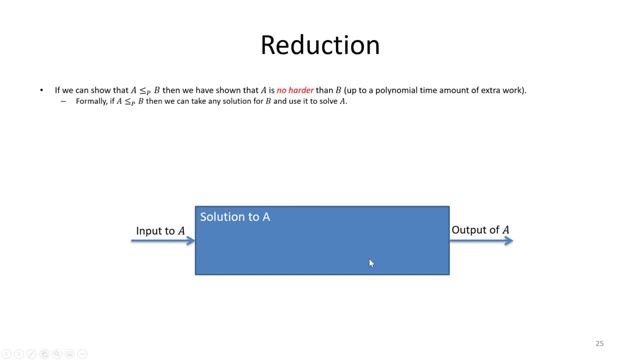 of the box comes outputs. So again, we're going to assume that we've got a decision problem here. so our outputs are just yes and no. You can think of that as a yes light and a no light, if you like, And what I'm going to try and show here is that A is no harder than B, by showing how. 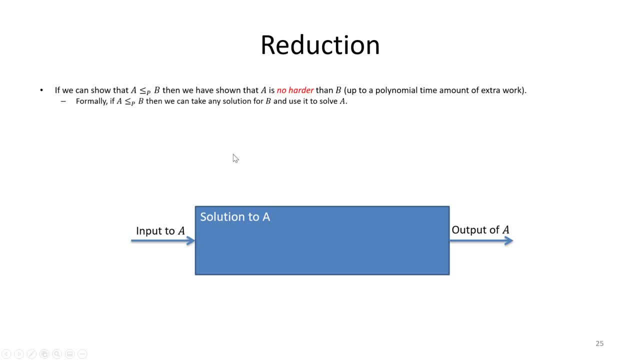 I can come up with a solution to A by using a solution to B, assuming we have this reduction. So we are going to assume we have this reduction and we're going to show how we can use any solution we might have for B to solve A. So what we're going to do is we're going to take 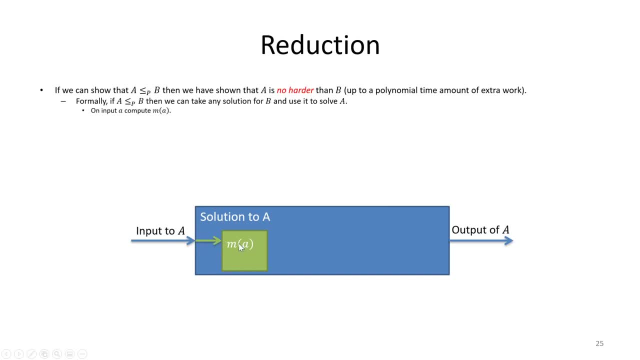 our input to A as it comes in and we're going to put it through our mapping that we get from this reduction M of A And remember what that does is it creates an input to problem B. So we're going to take that input to problem B and we're going to take it and put it through some solver. 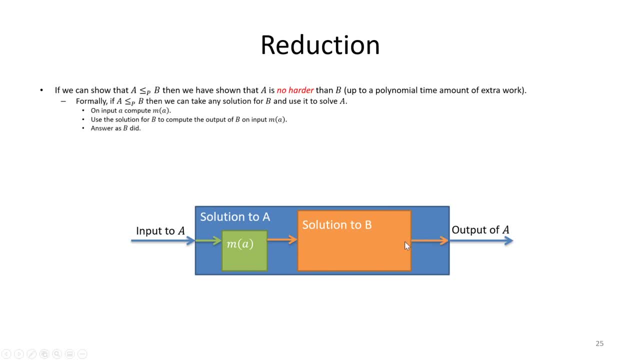 to B that we might have and then take whatever output B creates here and just answer that output as A, because we know that this mapping here M of A preserves the output, that if we were supposed to say yes on the input that came in, 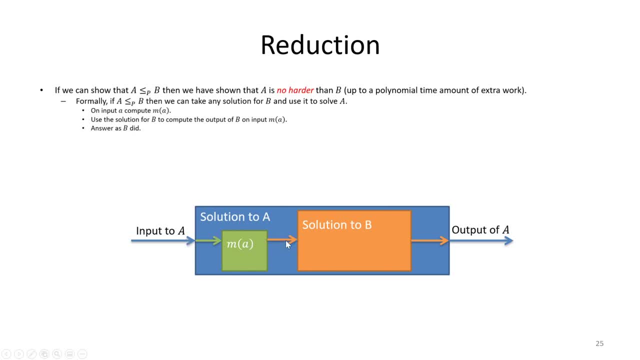 Then the input that comes out, the input to B that comes out of our mapping, would also be a yes instance, meaning after we put it into the solver for B, it will say yes and we will say yes, as we're supposed to. 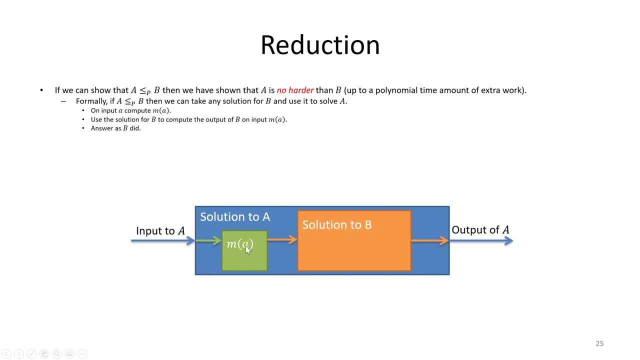 And the similar route for no. so if we were supposed to say no, this preserves that. So whatever input we create to B, we know the solver to B will say no on. so we will say no when we come out the other end. 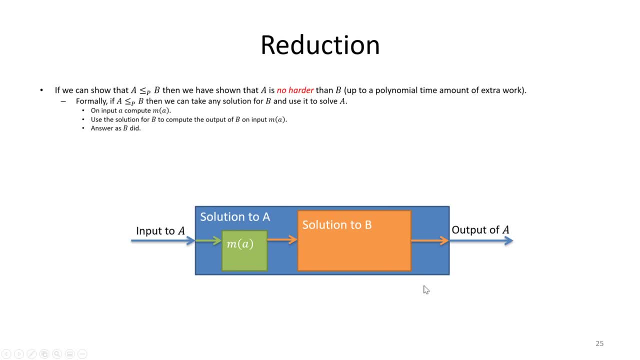 Now This diagram is sort of a map on how we can create a solution to A out of a solution to B. So when we want to consider the resources used to solve both, we can now have a solution that shows that any solution to B that we have say we come up with a better one one. 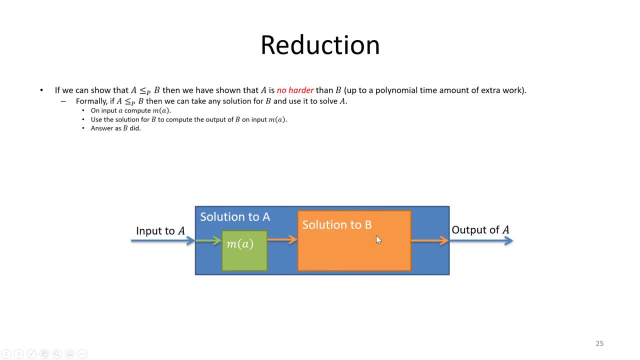 that solves it faster. well, we could take this, unplug it like it's a little circuit in a circuit board and plug in the new solution and our solution to A gets faster, As long as the solution to B- this part- is sort of taking up the most of the work. 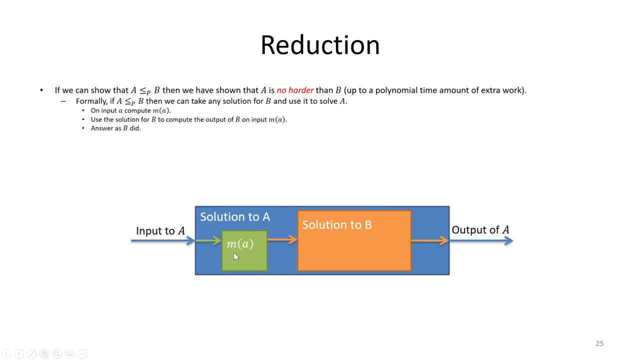 If M of A is really slow. this is where the polynomial time computable comes in. Let's say, M of A takes a lot of time. well, maybe that dwarfs. well, let's look at it a little bit closer. So we know that M is polynomial time computable. so this first step is going to take a polynomial 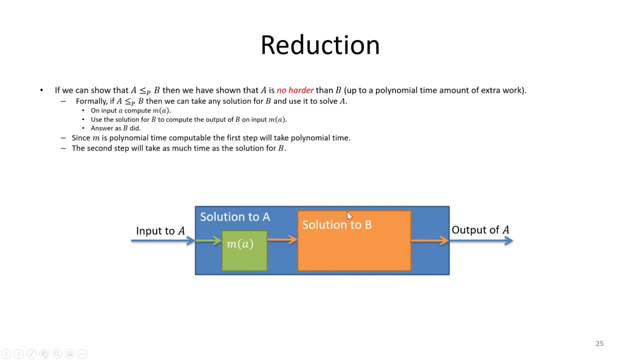 amount of time. Now the second time, the second step here. well, that depends on how much B it's going to take. however much time our solution takes, The solution for B is going to take, it only takes us a constant amount of time to return. 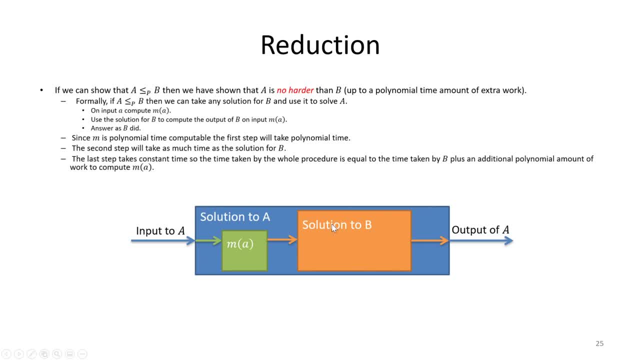 it so that the solution to A must be a polynomial plus however long it takes our solution to B to solve B. Now there's really two possibilities that I want to consider here. there's, of course, more than that, but there's two possibilities I want to consider. 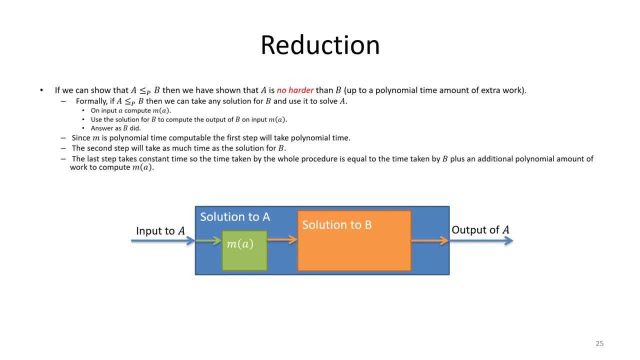 One is: our solution to B could either be polynomial time or not. So if let's for the moment assume that B is in P, so that we have a polynomial time solution to B, then knowing that A reduces to B, then putting this all together, that 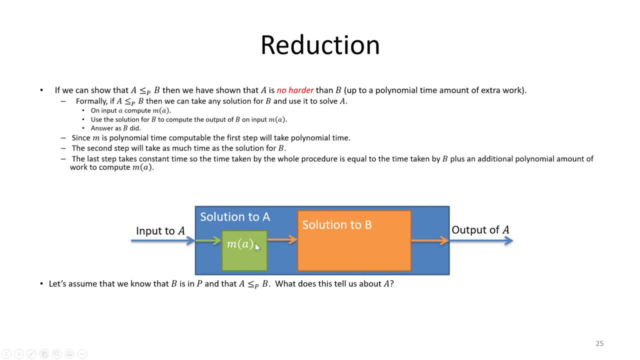 is, the total run time of A will be a polynomial amount of time to compute M of A, then a polynomial amount of time to compute the solution to B. A polynomial plus a polynomial is always a polynomial. So that means that The total run time for our solution to A must also be a polynomial. 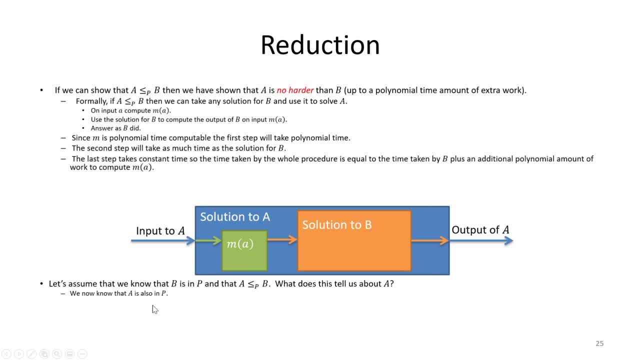 That means A is in our class P as well. So this seems to be one tool we could use for reduction and it's sort of the tool that you know a normal standard programmer might use when trying to solve a problem. If they identify a problem and say, hey, this problem is really really close to shortest. 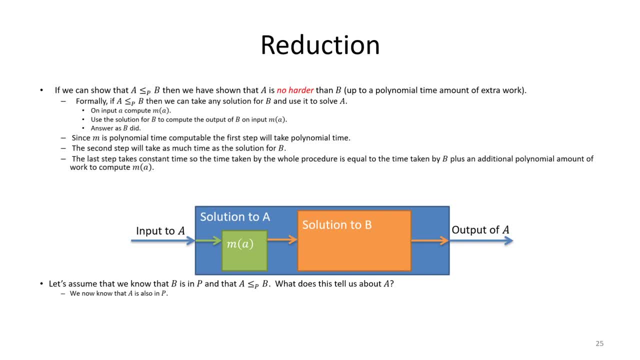 path, so I'll use Dijkstra's algorithm. or this problem is really really close to minimum spanning tree, so I'll use Prim's algorithm. When you recognize that a problem is very similar to another one and then you transform it slightly, you change it so that you can apply that other algorithm. you are effectively. 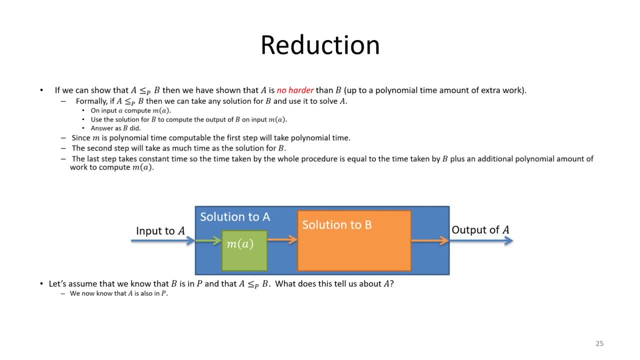 performing a reduction. Now again, you might do this in your normal programming and not think about it. it's sort of natural as a problem solving technique to reuse solutions that we have before and then. In fact, most of the strategies I've tried to address in this series of videos have all 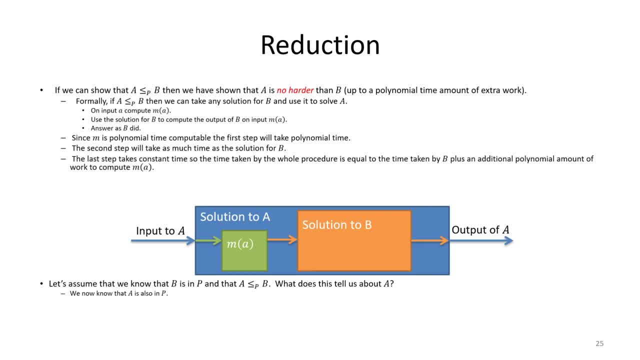 been exactly that: cases where we recognize similarities between how we solve problems and we try and reuse those solutions over and over again instead of reinventing them every time we encounter them. So this, like I said, this is one of the standard ways that we might use a reduction, but we 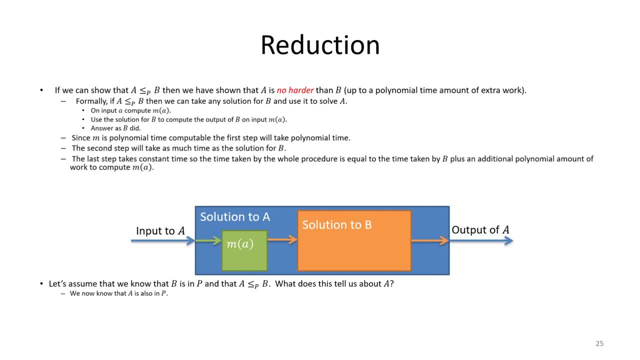 don't usually formalize it in this sense, We don't usually write a proof or something. The proofs usually come in when we want to use reductions for a different purpose, and that's sort of more what I want to explore now. So how can we use this further? 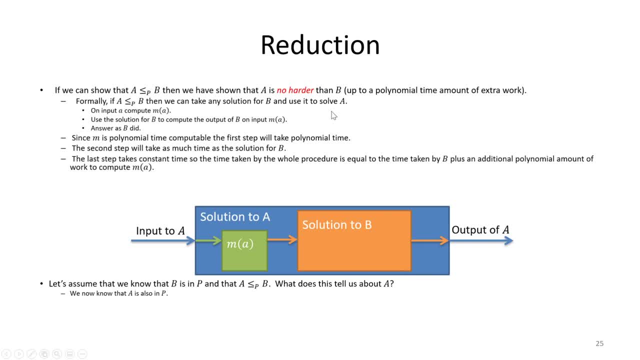 So the main takeaway here is that this less than or equal to really kind of means no harder than Now. it kind of looks like the solution to A is harder than because it's whatever solution to B takes plus something right. but remember, here we're rounding off stuff we're ignoring. 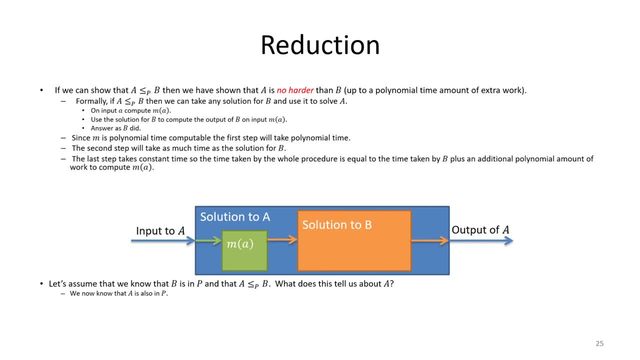 constants. we're even lumping all our polynomials together, so by sort of blurring our eyes a lot, the sum of these two together becomes effectively the same thing. We like to think of the green box as almost nothing, or at least dwarfed and certainly. 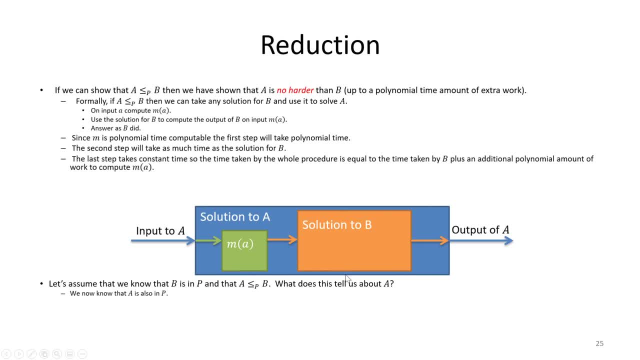 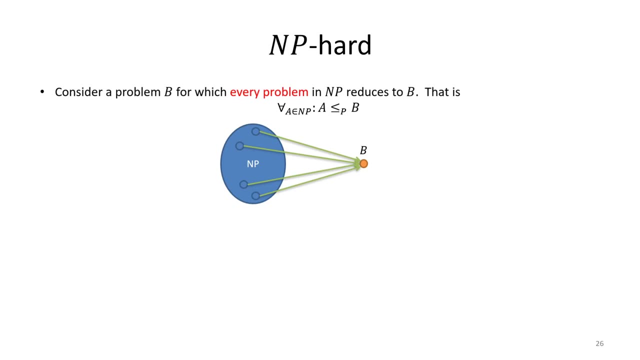 the other case, where B is not in P, where our best known solution is exponential, this is taking way, more way, much more time than just the mapping that we have here. Okay, let's consider another way we can use our reduction here. So the next idea that I want to encounter here is: I want to take you sort of on a thought. 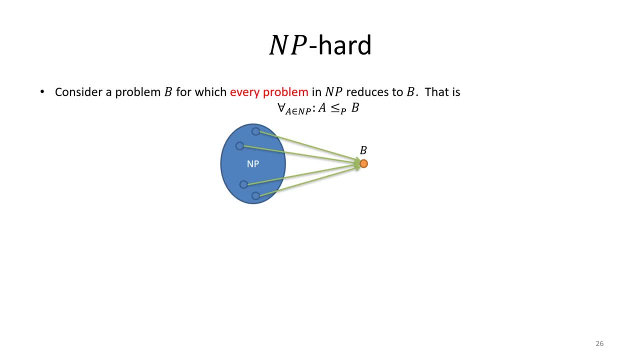 experiment. I'm going to make up a problem here that you don't really have to believe exists, but for the moment imagine it exists. So imagine we have this problem B here, that every problem in NP reduces to B. so using a little bit of logic, 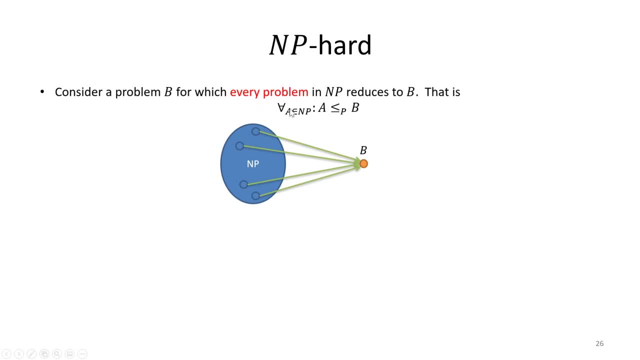 A little notation here. this is for all of the problems A that are in the set NP: A reduces to B. Okay so imagine that this problem exists and I've sort of just depicted this pictorially with these lines depicting our reduction. 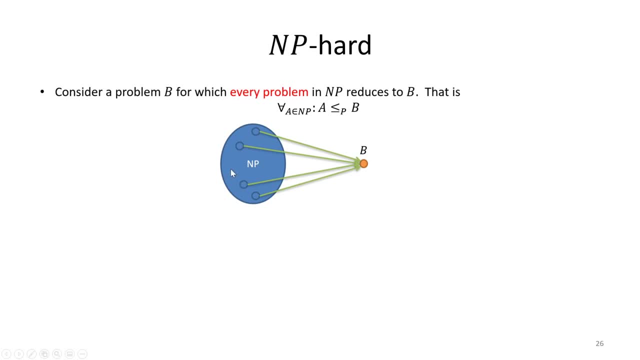 Here's our special problem B and here's all the problems in NP reduced down to it. So remember that this means that A A less than B, A less than or equal to B means A is no harder than B. Now that means these problems in NP. 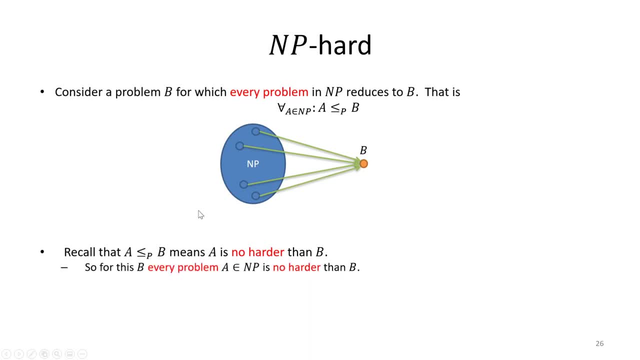 are no harder than B. Now another way to say that is that B is harder than these problems, although the no harder part means it's possible that B is equal in difficulty to some of the problems in NP. We know some are really easy, some are harder. but if there's a hardest one in there, B could. 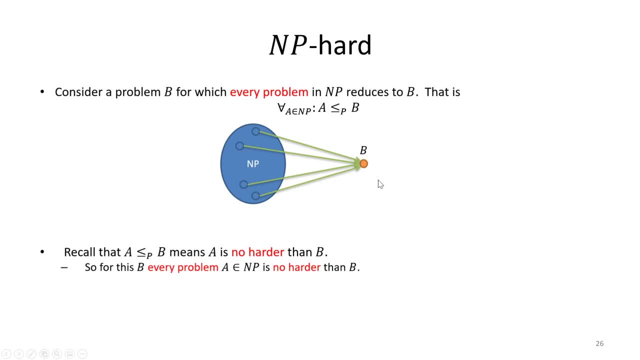 be potentially equal. At least this is the relatively simple pattern. Then you can round off and call it B. but if you were gone down to B, it's not咒n yow, you would haveöttan for 6.. 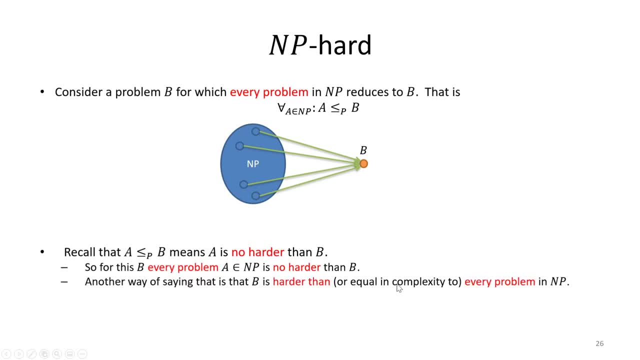 So just this is where I've kind of put a here or equal in complexity apparent factor in terms of the problems in NP. Remind us that it is also implied here, but it is sometimes make it a little bit easier in this step. well, B must be harder thenashore than the problems in NP. 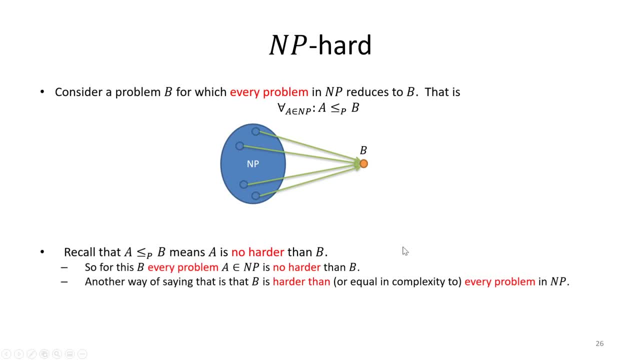 And it very well COULD be harder. it very well could be much harder then the problems in NP, At least as far as we know, B this problem B if it existed, it seems to represent a pretty hard problem. all the problems in NP are no harder than it, so this is harder. 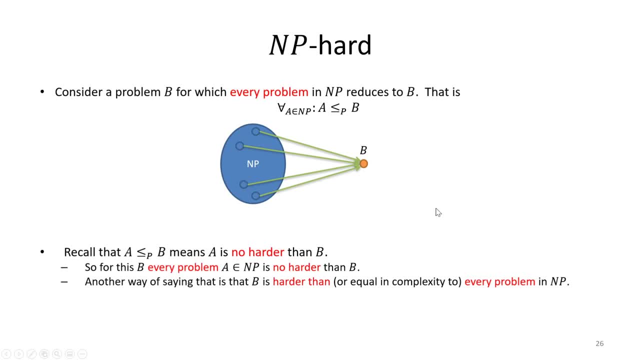 than all the problems in NP, or at least most of them, and so we're going to define this class now here that I'm going to call NP hard- or that's what it's been called, of course, in the literature- which is basically all the problems that have. 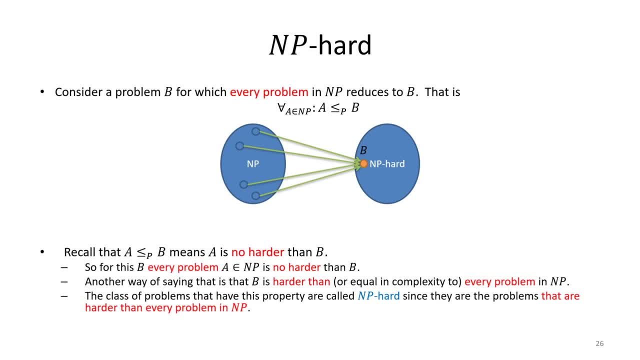 this property. so if you could find a problem B such that all the problems in NP reduced to it, then we could call this problem NP hard. okay, now you follow me down my fairy tale, imagining that this, this problem exists, or that this class of problems exists, but you really, at this point, have no reason to believe that this problem. 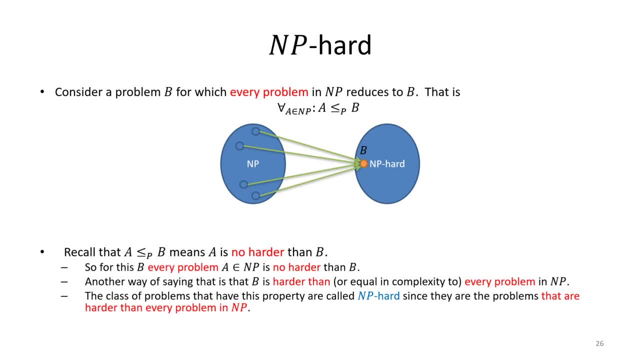 exists or that this class of problems exists or is not empty. it certainly can exist and be empty. so let's consider this a little bit. how can we show that there's such a problem? B that has this property? well, first of all, on face value. if we just try and prove this statement here, we could use our definition of a. 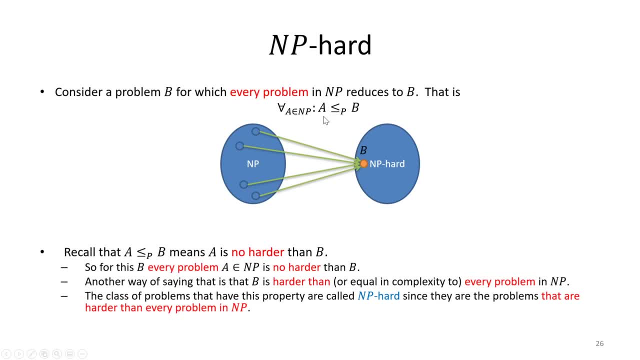 reduction that we just looked at to try and find mappings from problems in NP to this problem and we could maybe think, well, we have, it's a for all. it means we have to do this for all of them, which means we might go through. we've had- we have- a couple candidate problems already. we've. 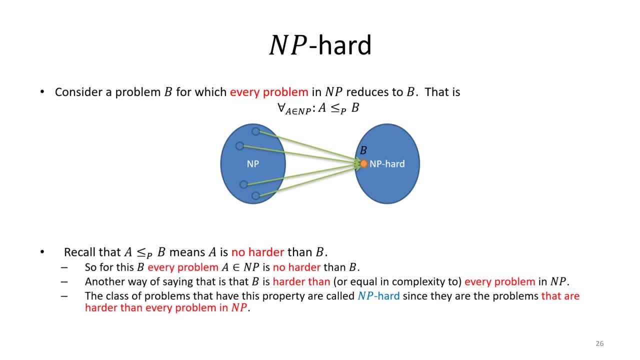 got. you know the composite problem we showed. that was in NP. we showed subset sum partition knapsack. we showed that clique and independent set and Hamiltonian cycle. all these problems we've shown are problems in NP so we could go one at a time and try and reduce them. now that 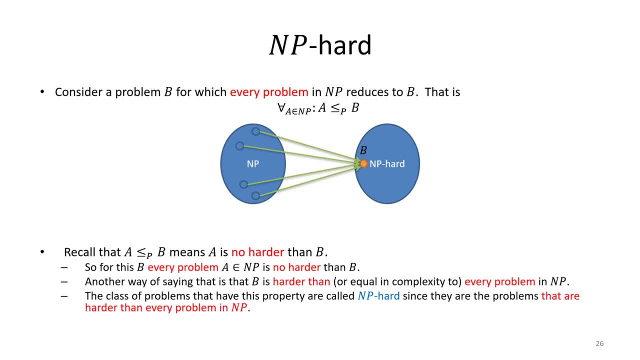 already sounds exhausting to me. I don't really want to engage in that. the %um, one of those proofs, is probably challenging enough %um. and then, even if we started on that path, we might stop for a moment looking on the policy. how long is this time? how many problems are there? 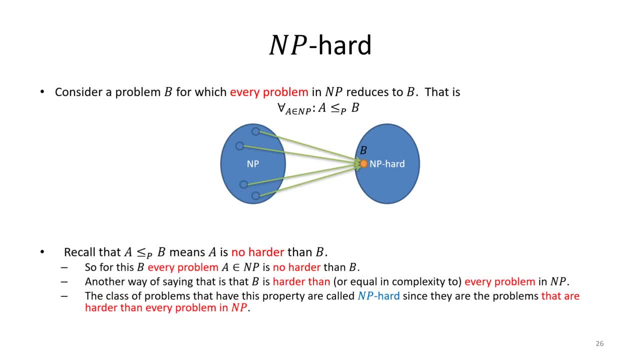 in NP and we might realize that how? there's the day, there's infinite. problem took a piece 0? well, this path is certainly not. we're not going to get anywhere if we start down so, but you might have even more reason now to do that this problem be exist. 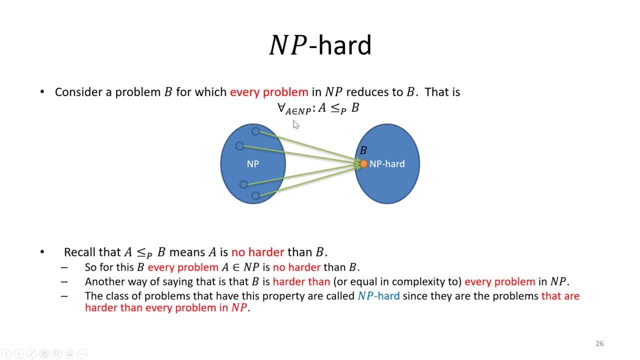 it exists. we would have to prove this statement for infinite values of A. infinite problems, A? okay, so imagine still that we're able to do that. someone's able to do that. okay, again, bear with me for a moment, spoilers. someone was, but follow, follow through with me in a second. okay, so now. 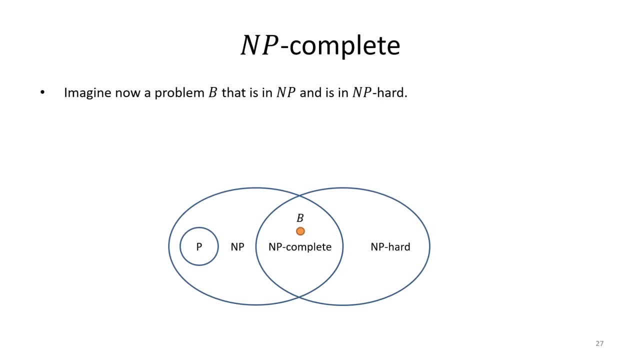 imagine that the problem B that we have is itself a problem that we can say is an NP, so we can give a verifier for it and and prove that it's correct and runs a polynomial time, then we know that problem is also an NP. so if we have this, 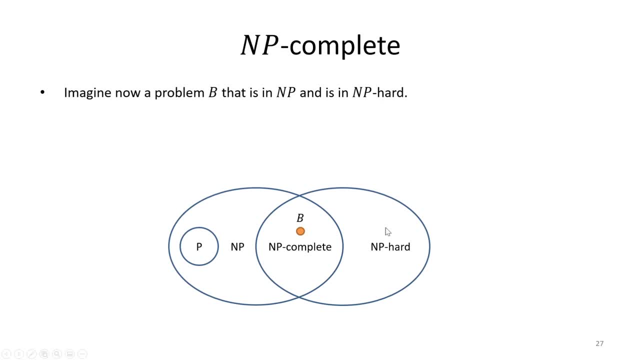 special problem. it would be, because it is an NP, hard. it would be harder than or maybe equal in complexity to every problem in NP, because it's in NP. we know it's not harder than itself, so it must be equal in complexity to itself. then it must be the 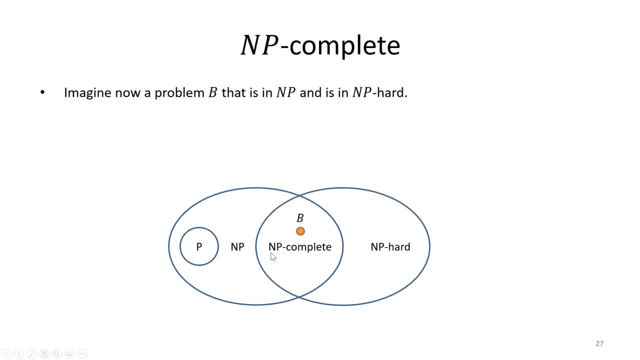 hardest problem in NP and if it is the hardest in our problem in MP, you were going to give a special name to that. we're gonna call it NP complete. and it turns out there's not just one such problem, there's not just one hardest problem in NP, there are a lot of them, there are hundreds of them that we are 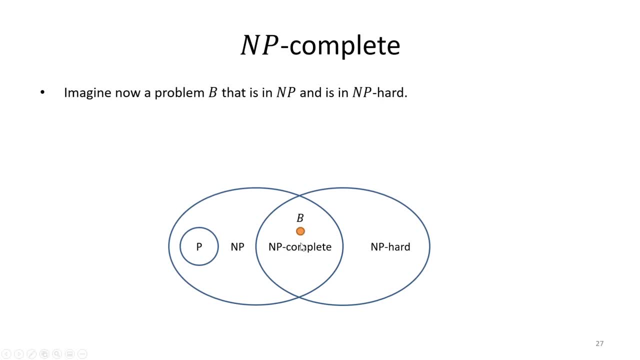 aware of. there is potentially infinite of them, but there are a hundred sort of real-world problems that we know or NP complete, and all of these problems represent a problems in NP. Now, remember what we were looking at earlier was the idea that we could, if we have this reduction from a problem to another, then that might be. 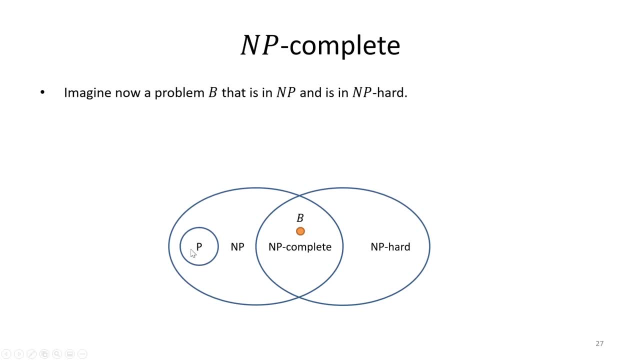 helpful in showing that a problem is in P. If we had A and A reduced to B and B was in P, then A was in P too. The reason we're focusing in on this hardest problem in NP is if we want, if we're coming up with a strategy to show that. 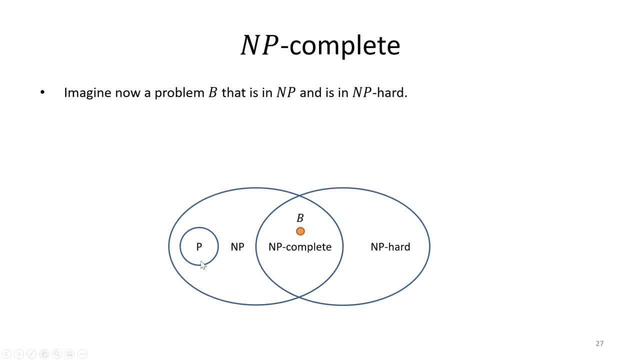 all the problems in NP are also in P. our best strategy might be to focus on this problem, the hardest problem. Okay, so I think I mentioned this. so B is an example of the hardest problem in NP, and again, we call these NP complete. Now here's this strategy that I was looking at here. so imagine we have a problem. 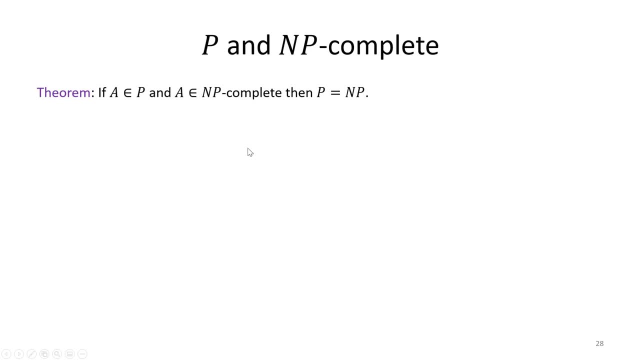 that's in P and it's NP, complete. I'm going to argue that if that were the case, then our two classes collapse. Now remember, this is an open problem. we don't know if P is equal to NP, so we don't know if this first part is true. but let's follow through So. 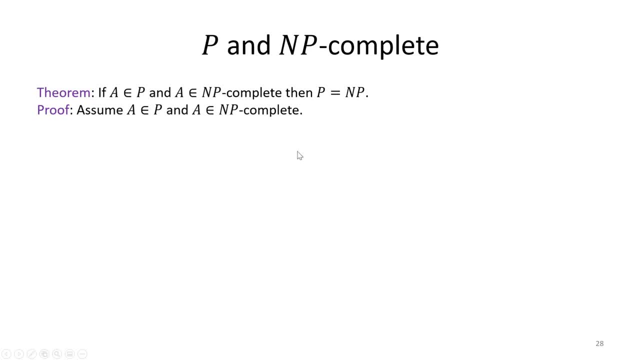 assume A is in P and assume our A is also NP. complete Now, since A is in P. what do we know from that? Well, the definition of P says that we must have a polynomial time algorithm, deterministic algorithm, that solves this problem, A. So we know this from our definition here of A being in P. 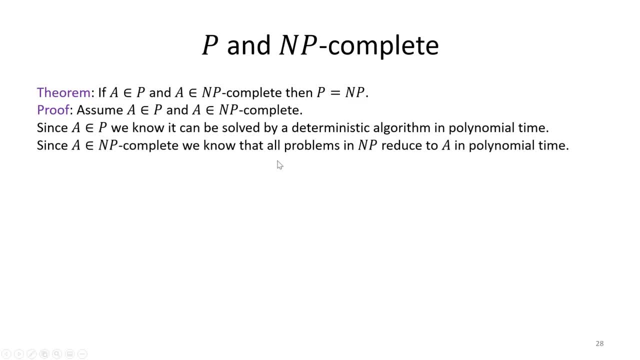 Now what else do we know? If we know that A is NP-complete, then we know that all the problems in NP reduce to A in polynomial time. Now, specifically, we know that because A is NP-hard, but NP-complete implies NP-hard, And so what we get now is that any problem in NP, since they all 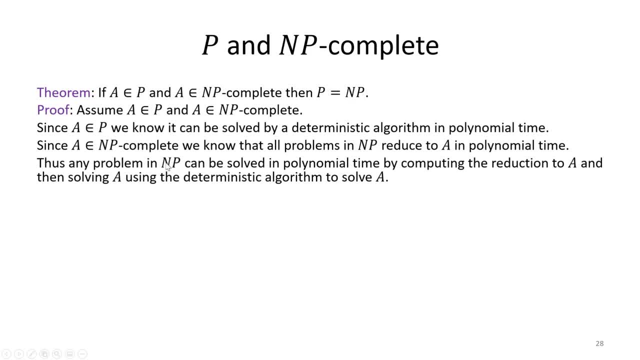 reduce down to this problem A that we're considering. okay, all of those problems can now be solved in polynomial time by doing a two-step process. We will compute the reduction that we know exists from it being NP-complete. That takes polynomial time, And then we'll use 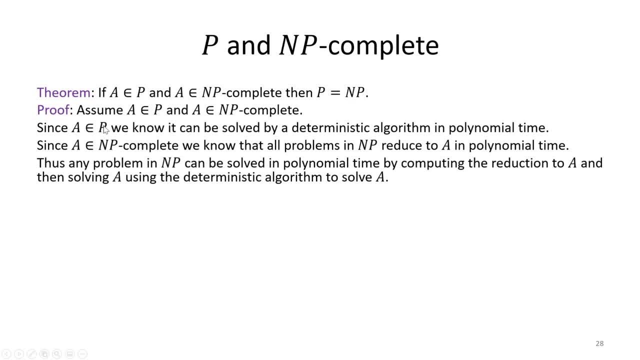 the polynomial time deterministic solution that we have for problem A to solve A. Remember, because our outputs are preserved here. this will ensure that we solve what you, whatever problem in NP that we're considering, And so our problem in NP is now polynomial time. 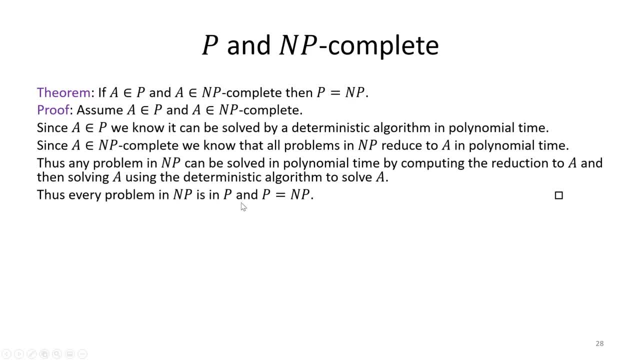 solvable. Therefore, every problem in NP is NP and P must be equal to NP. Now the last bit. I haven't included the fact that P is a subset of NP, but we proved that in a previous video. So this we're filling in the last bit, the relation that NP is a subset of P. So all we need to do. 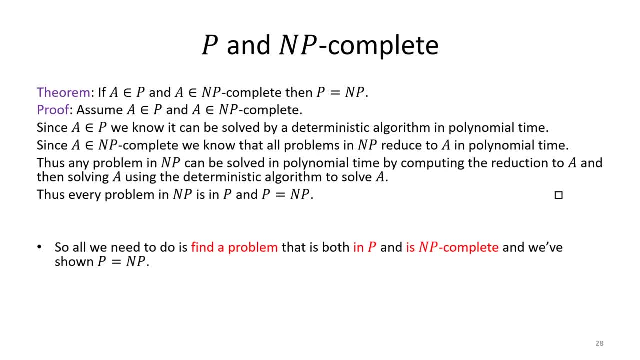 if we want to prove P is equal to NP is find a problem that is both NP and is also NP-complete. Now I say all we need to do. It sounds like it's an easy thing to do but of course- and we know of problems in P, we know of problems in NP-complete. We'll prove a couple here in a bit. 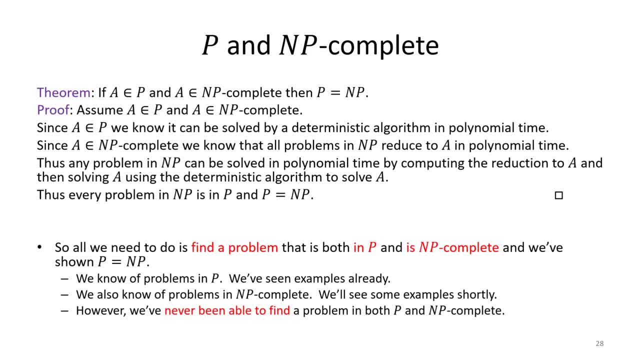 However, all of complexity theorists and computer scientists, since you know, 1971-ish, when this, when this question was first posed, none of us have been able to find a problem that satisfies both of these criteria. And that's a lot of us. A lot of us have tried. I've tried too. 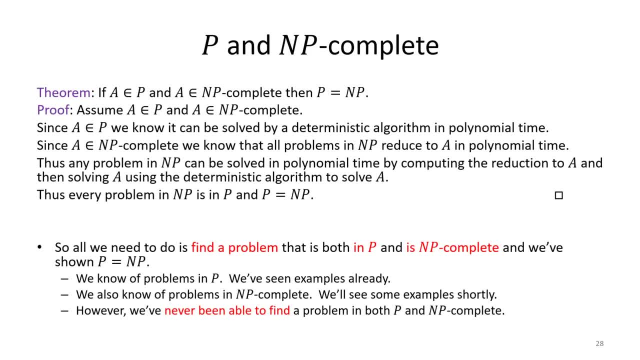 None of us have found it so far. That doesn't mean that such a problem doesn't exist. It just means we have not been able to find it thus far. However, those of us who have worked on it, if you search for a very, very long time and fail to find something, 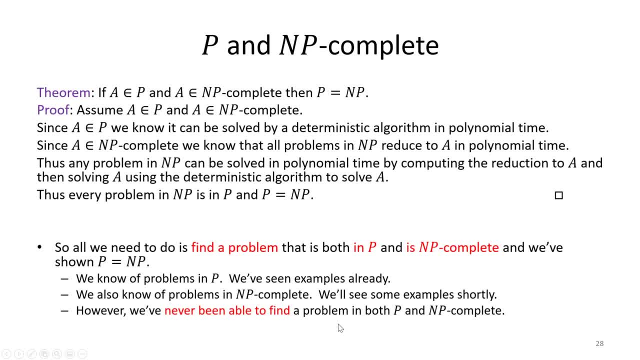 you start to build up a confidence that that thing does not exist. That confidence is built on nothing other than your own failure, So it's not. it's not an evidence-based confidence, But what it means is some of us who have been have worked on this for a while, and 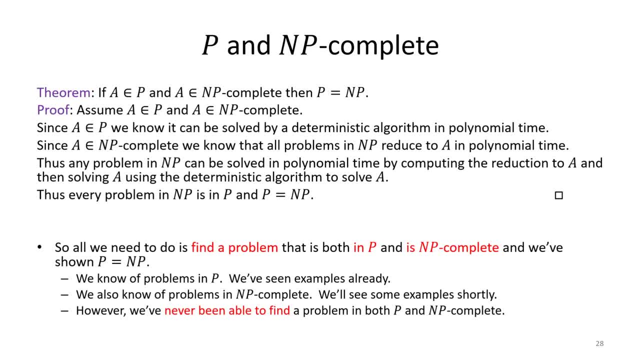 have sort of considered the problem for a while, we maybe have lost the ability to come up with clever new strategies on it, And it's really up to someone who isn't so convinced by their own failure that this is impossible. So I do always encourage. 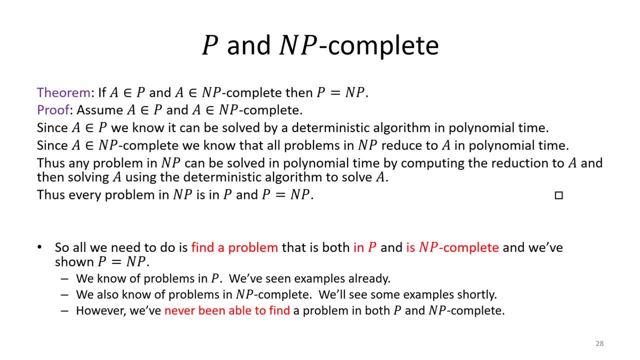 you know, younger researchers, new researchers, go out there and try something new. Every year there's a new surprising result: that some young researcher somewhere says, hey, I haven't tried that before, Let me take a crack at it. And you know, a couple of weeks later they say, really, that took you guys. 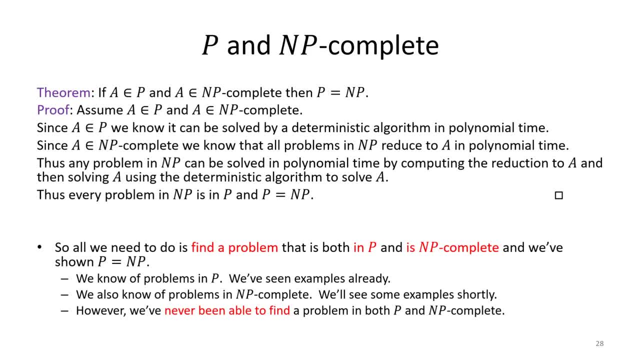 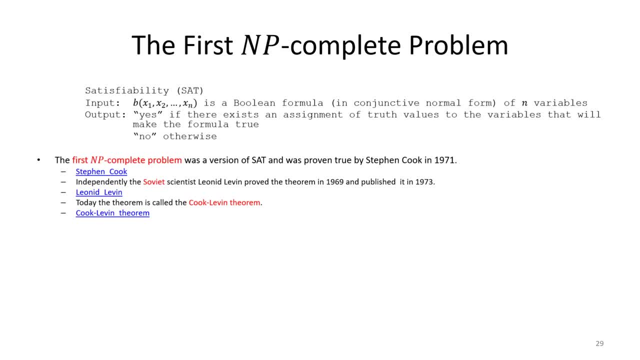 50 years to solve. It took me. it took me a handful of weeks. So maybe that's you, So try it out. Okay. so to continue our storytelling, I want to say, okay, what was the first NP-complete problem? 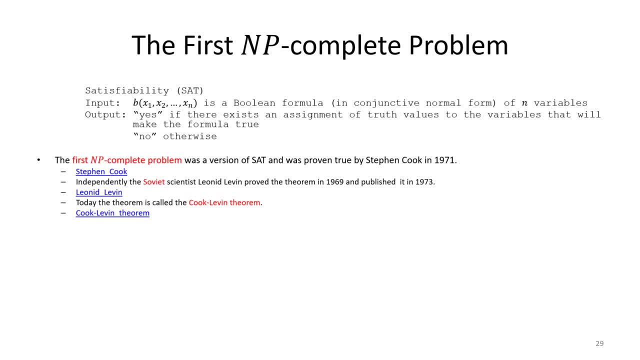 So the first NP-complete problem is this one here: Satisfiability. And maybe I'll take a moment here to just talk about satisfiability as a problem. First of all, it's an interesting problem. It's a logic problem. It's a problem where you get a Boolean formula. 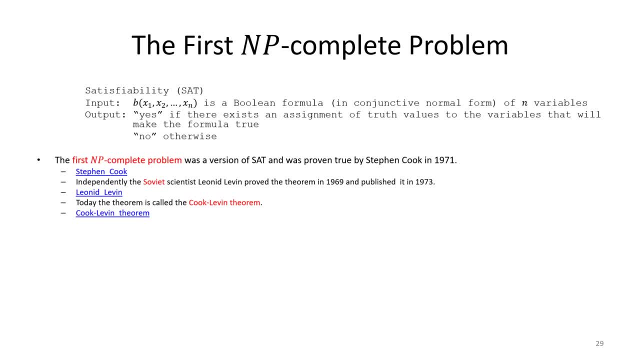 Now if you need to recall back to your logic class, for what a Boolean formula is, Boolean formula is a formula of Boolean variables, first of all Variables. here I've got indicated x1,, x2, xn. Now a Boolean variable, of course, just like a Boolean variable in a programming language, is just a true-false. 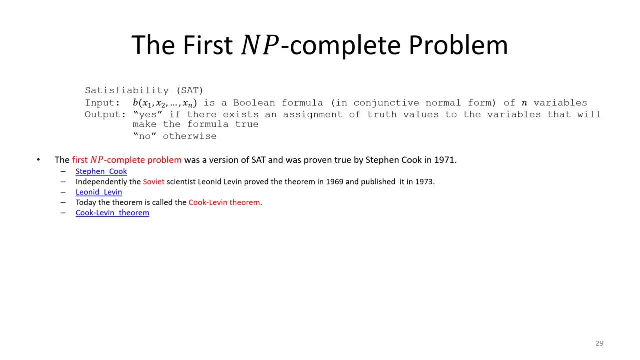 So each of these could be assigned a value, either true or false. but the Boolean formula is joining these variables together using standard logical connectives like ands, ors and nots. However, we're going to state here that, for our problem of satisfiability, 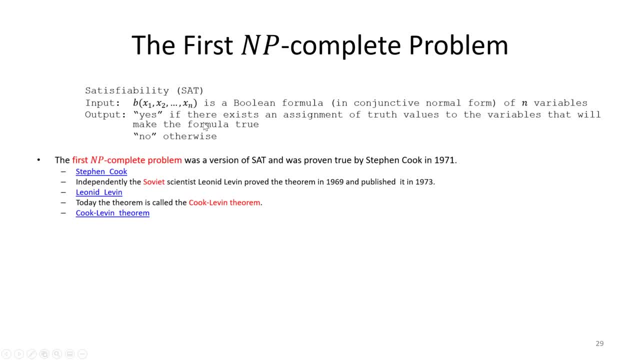 we want to convert that Boolean formula, at least for this problem, into conjunctive normal form, And then we want to answer yes, if there's some way that we can assign truths and falsehoods to x1 up to xn, so that the whole formula at the end becomes true. 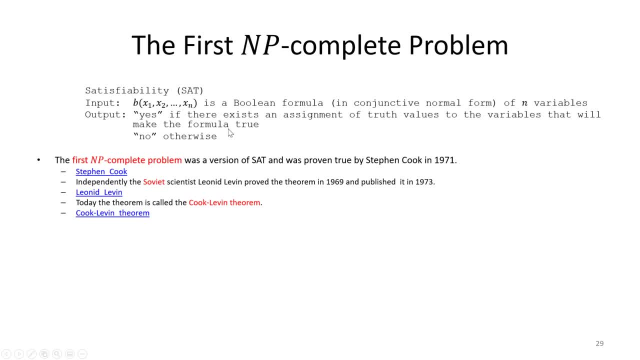 If there is such a way, we say that the formula is satisfiable. If there is no such a way, then the formula is a contradiction, meaning it's always false, And so this is sort of an important problem in logic and in computational logic. 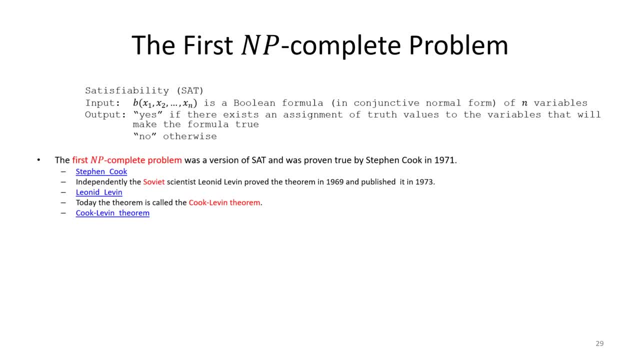 importantly. So say, you have a big, long Boolean formula and you want to know if it's a contradiction or not. So this problem actually is the first NP-complete problem for one important reason, and that is that because it is a logic problem and it has an important parallel, 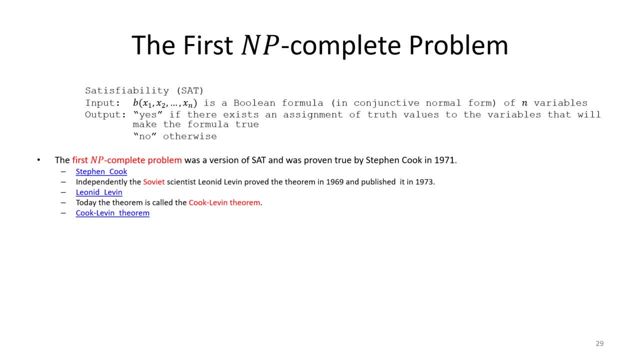 as we'll see in a second to NP problems. it really stands out- It's sort of the quintessential NP problem. It really stands out as a good representative of NP- and we'll see that in a second, But this problem was the first. 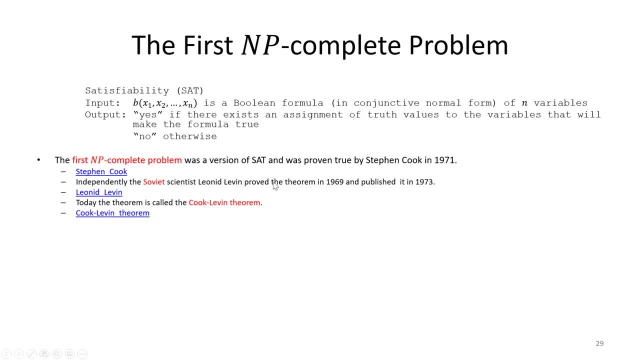 NP-complete problem and it was proven independently by two researchers. as was somewhat common at the time during the Cold War, researchers in the Soviet Union and China and so on were isolated from researchers from the West, who likewise were isolated from them. So 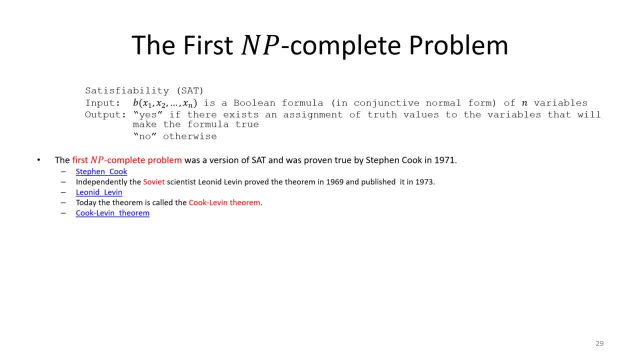 research done in one of these spheres was not always shared with the others, and so it wasn't until sort of after the end of the Cold War where we realized: oh, this same result was actually proven twice by independent researchers, And actually it was proven around the same time. 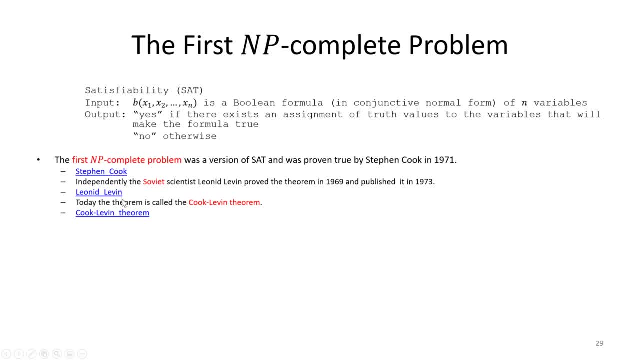 the early 70s by both Stephen Cook and Leonid Levin. Now Stephen Cook participated in the sort of Western publication realm, and so he published in 1971.. Leonid Levin proved the theorem sort of privately in 1969 and then published it in 1973. 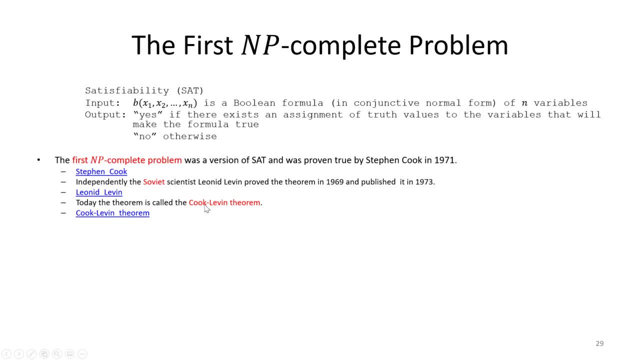 And so today the theorem is named after both of them. We often call it the Cook-Levin theorem and you can find more information about them and the theorem on Wikipedia. Once again, they're famous for proving that this was the first NP complete theorem. 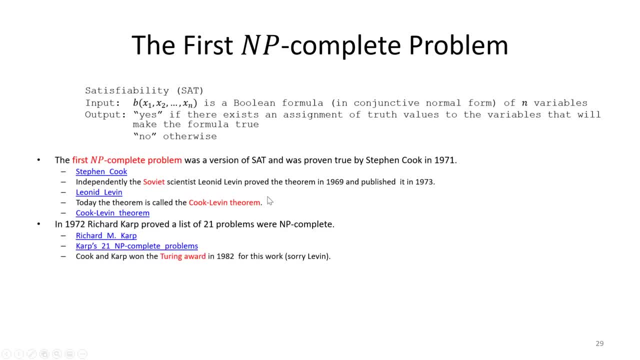 which was a daunting task. but after they were able to do that, quite soon after, actually in 1971, or sorry, in 1972,- Richard Karp was able to expand the list of problems from this single problem to a list of 21 additional problems. 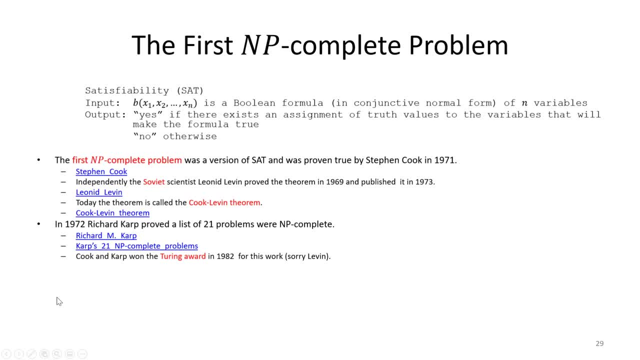 of problems, from this single problem to a list of 21 additional problems, problems. And so actually in 1982, the Cold War was still on. so sorry, Levin, but Cook and Karp during that time won the Turing Award for effectively founding the field of complexity. 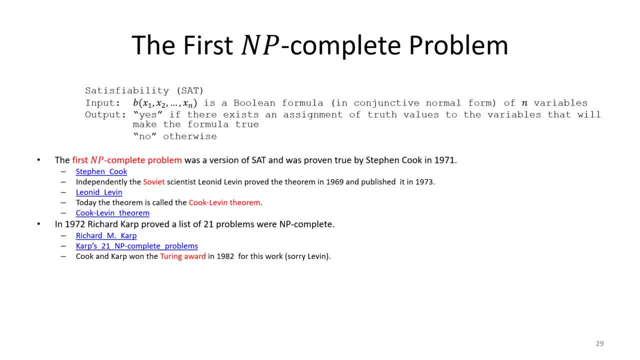 theory and posing the first open question in the field, which was: is P equal to NP? Which here we are, 50 years on, almost without an answer to that open question. And then, after that, the field had been founded in 1979. A pair of researchers named Gary and Johnson published a book, a fairly famous 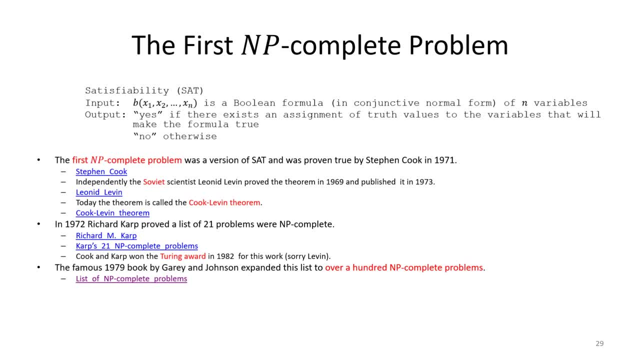 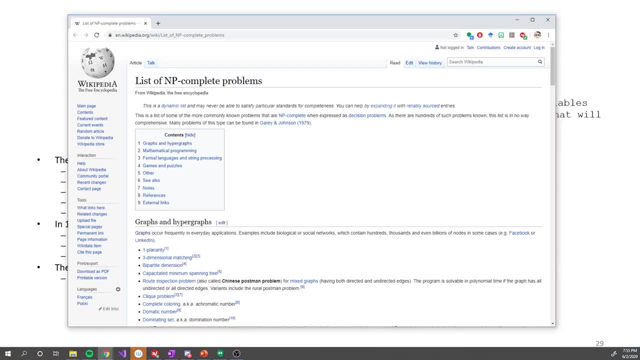 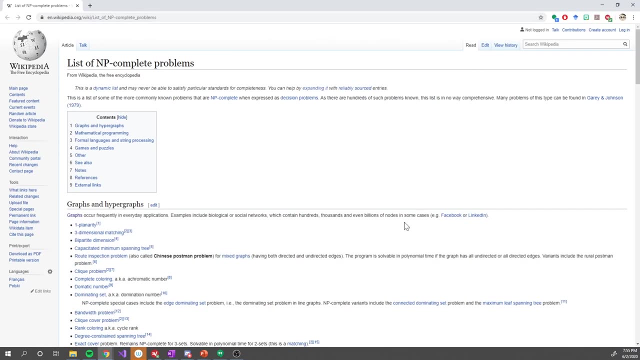 book with over 100 NP complete problems in it And this book is actually sort of worthwhile reading if you're interested in NP complete And I've actually got here just the Wikipedia page only to take a look here. This is the Wikipedia page of the list of NP complete problems And we could maybe spend some time looking at. 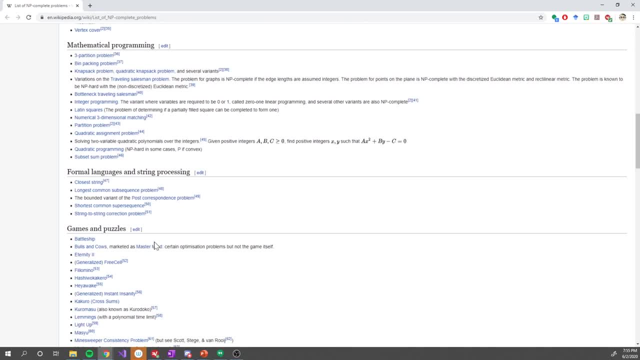 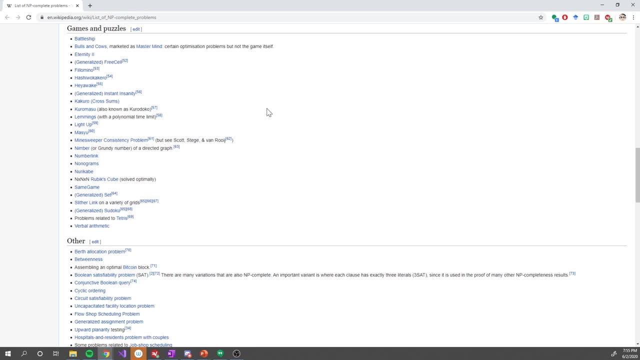 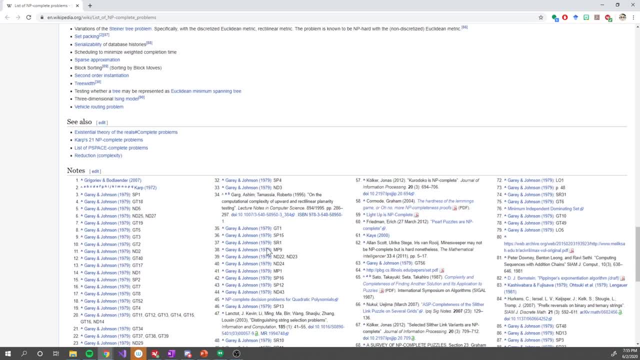 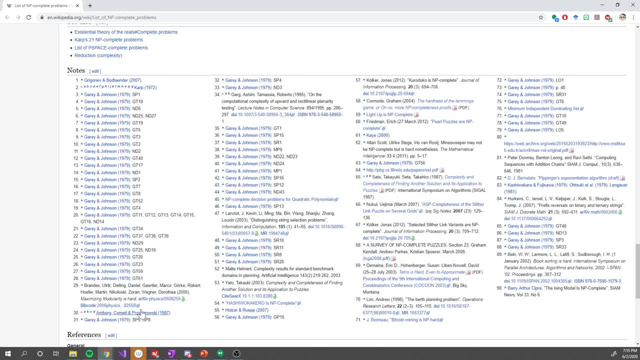 So N can grow largely Other interesting ones that go on. but the reason I kind of wanted to show this was mostly just to show the reference section and show you know how many of these proofs, how many of these reductions, were actually first shown in Gary and Johnson. 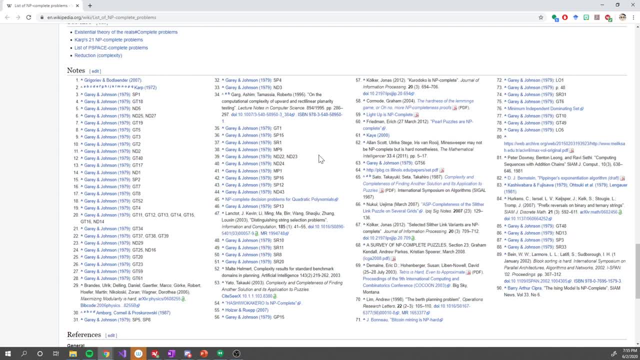 In Gary and Johnson. I actually studied complexity theory in some detail during my Master's degree And I do remember spending, you know- afternoons and hours of work, you know sitting in the library reading Gary and Johnson, reduction after reduction, and some of these are really interesting and clever reductions, and some of them are. 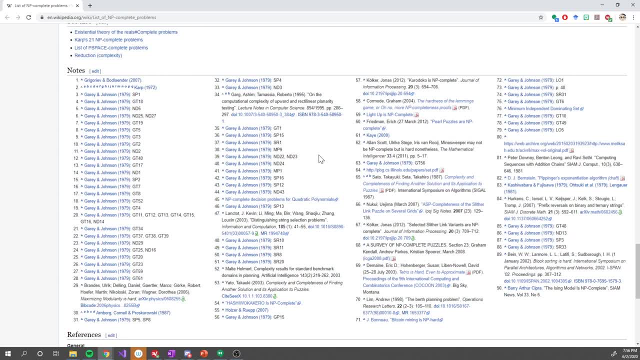 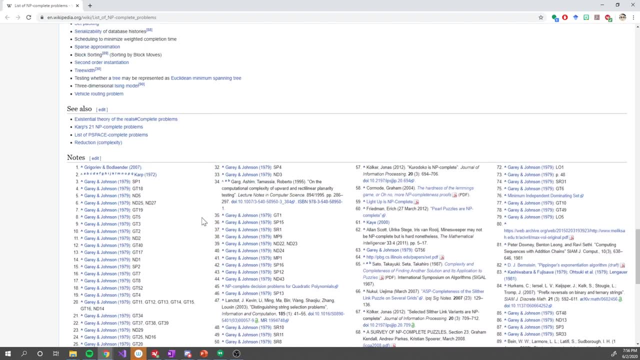 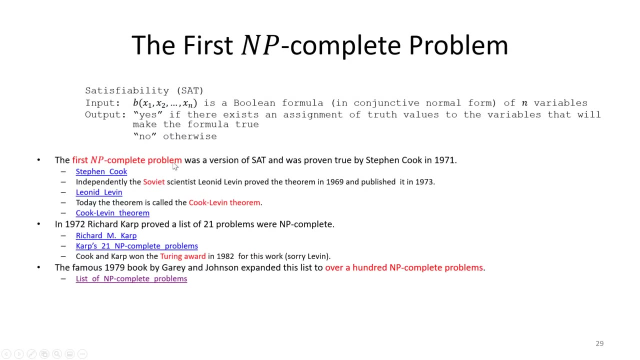 proofs that take several pages, so it's not exactly. it's pretty dry reading, but if you really like mathematical proofs, dive right in. it's a fun book okay. however, I bring it up here mostly just to tell a little history story of the expansion of our list of NP. complete problems and since 1979 we continue to. 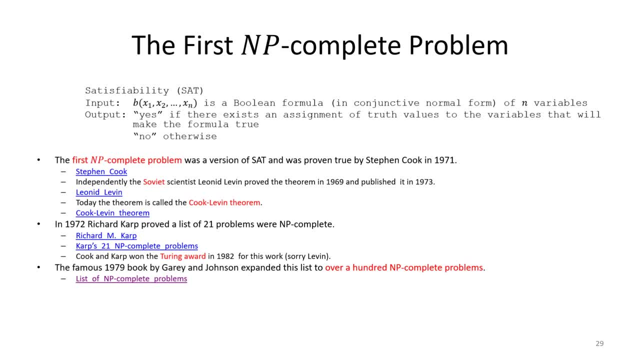 add NP complete problems to the list. every once in a while we encounter a new problem that maybe is caused by a new kind of technology, but more often than not there's some grad student who needs a thesis and they say, oh, you know, Pokemon is NP complete, or something like that, and they'll go prove. 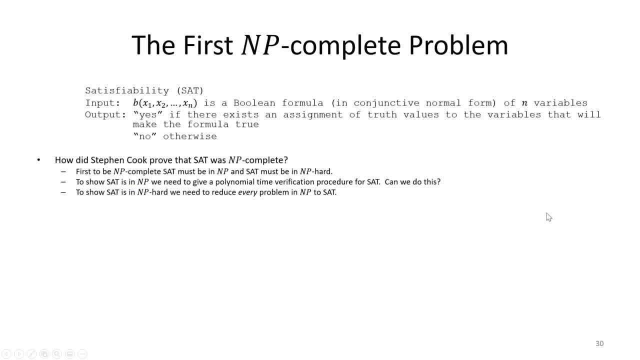 it so that they can earn a degree okay. so I want to talk a little bit more about the strategy then behind it. how did Stephen cook and and Lena 11 prove that's that was NP complete? well, they actually relied on a concept due to Alan Turing called a Turing machine. that. 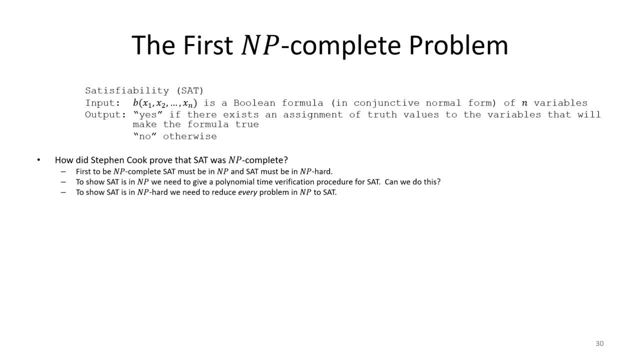 makes makes it a little bit easier, then, then I'm gonna attempt to approach it right now. but the way that we can do this is so: first of all, we have to address what is it the task at hand? we need to show that every single problem in NP can reduce to SAT, and so to do that, that seems. 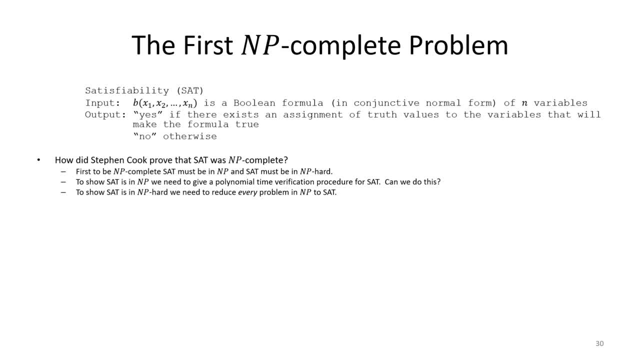 daunting. as I mentioned, there's infinite such problems and on top of which we don't know anything about the problem. we have to grab the problem. so one way to do infinite problems at once is to make a general proof, start out and say we'll just take any problem in NP generally, arbitrarily, without knowing anything. 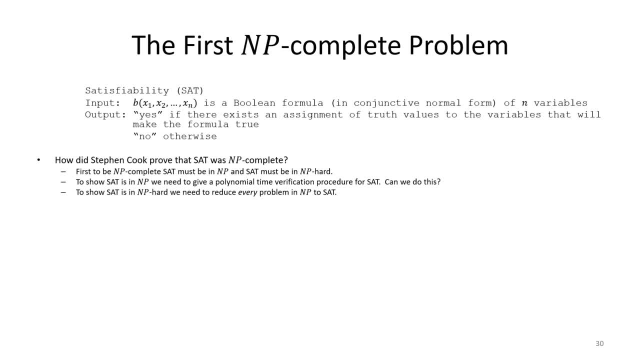 about it, not one, not our favorite one, just any old one- and then try and show that that problem reduces to SAT. and that's indeed the strategy that they take. But what that means is they somehow have to find- and this is exactly what they're going to do- is try and take the definition of what it is to be an NP problem. 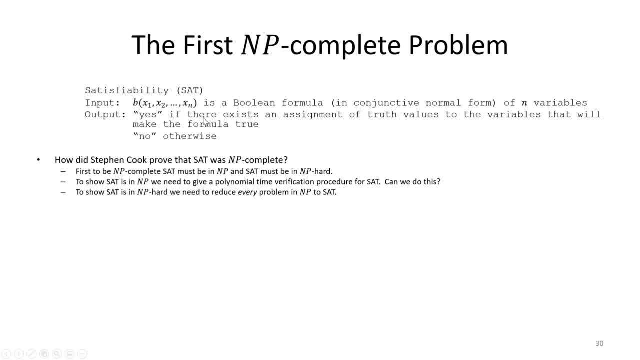 and express that as a logical statement. And that's why it was really important that the first NP-complete problem is a logic problem, because this logical problem has the same logical structure as our definition for NP. Now, what was our definition of NP? 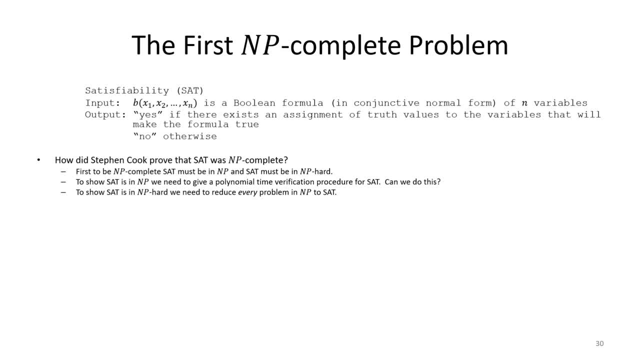 Now let's loosely dangle it out here. I'm not trying to write a full proof, because it would take us a while here, but the idea behind it is our definition for an NP. at least the one we've encountered is that you have this verification procedure, okay, And what that means is this: 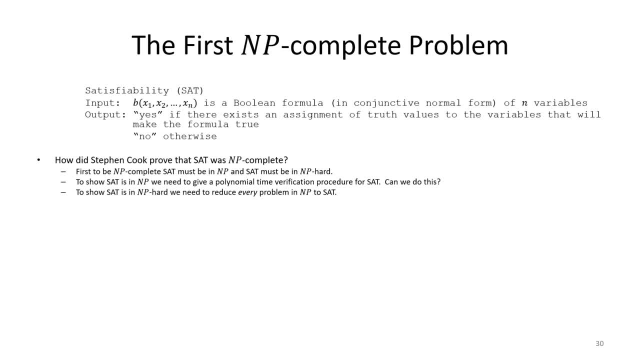 verification procedure. the way it works is: if we should say yes, then there exists a way that we can make it say yes, There exists a proof that we can insert into that algorithm that at the end it will say yes. And then also, if we're supposed, 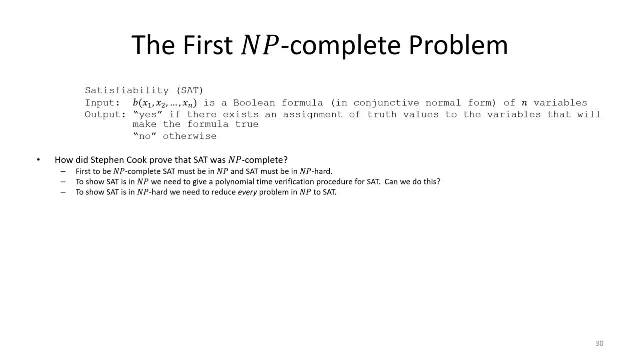 to say no, then no matter what proof we put in, we should say no. Now let's look at the definition of what it means to be satisfiable here. A Boolean formula is satisfiable if there exists some set of values. let's call it a proof that we could assign here. that would make 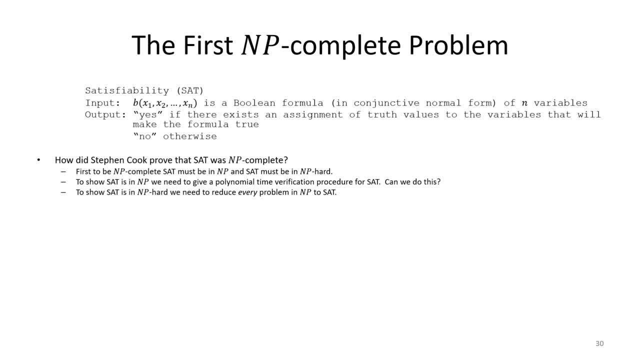 the whole thing true, ie say yes. On the other hand, it's not satisfiable, it's a contradiction. if every possible way we could assign truth values here, every possible proof leads us to no, And this symmetry between the definition of how a verifier works, what a correct 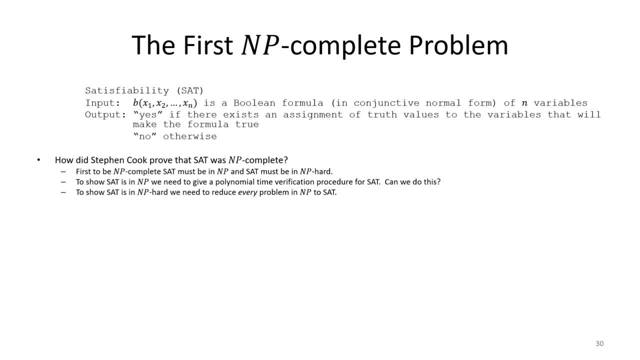 verifier is matches very, very closely the definition of what a satisfiable Boolean sentence is. And what that means is we can actually write that definition of the NP sentence, the definition of the NP verifier, down as a Boolean sentence. And that was the cleverness. 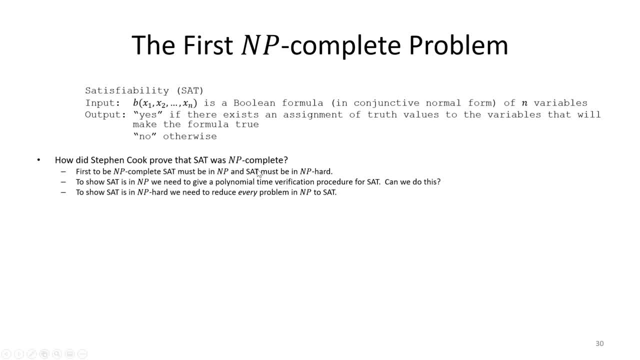 that Cook and Levin were able to come up with. In so doing, they were able to say that I don't need to know anything about the NP problem ahead of time, only that it has a verifier. and that alone is enough for me to show that there's some corresponding Boolean sentence that will say yes. 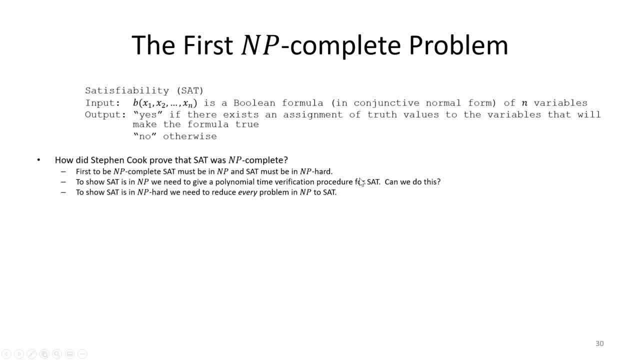 when it needs to and say no when it needs to as well. So, again, if you're interested in that, go take a closer look at the Cook-Levin theorem, But you may need some familiarity with Turing machines, depending on which version of a proof you encounter. Okay, so this was sort of a 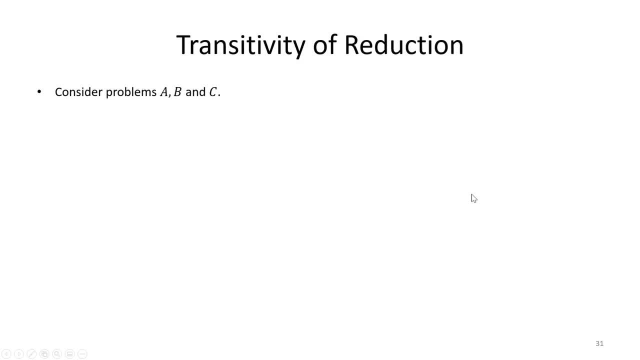 challenging problem. I think I've encountered this already, But let's move on and see what we can do. Okay, so this was sort of a challenging problem. I think I've encountered this already, but let's move on and see what we can do. 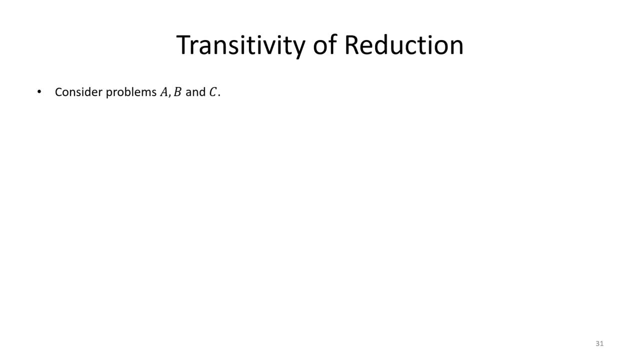 How, after they were very clever and were able to get the first problem, Karp was able to come along and grab a whole bunch more very quickly. Chen, we have some problems here: A, B and C decision problems still. Then, here I'm going to state: 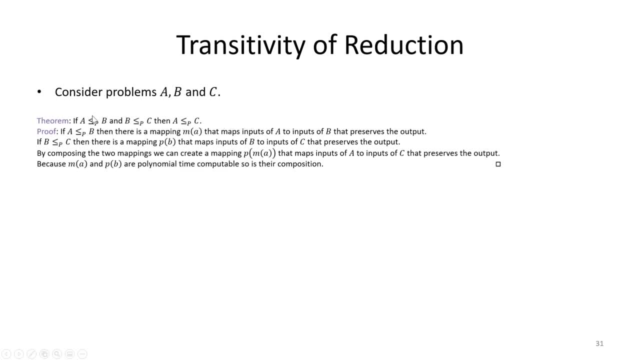 the transitivity theorem. This is true of numbers. so if A is less than B and B is less than C, that means A is less than C. We're just taking that property, the transitivity property, and applying it to our reductions. Here I want to prove. 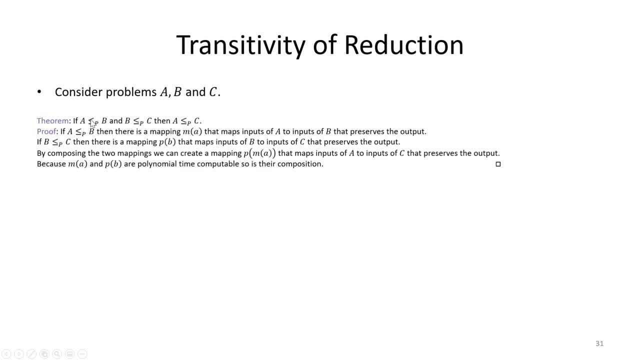 it to you. So we're going to start out by assuming the antecedent that a reduces to b and b reduces to c. Well, if a reduces to b, that means there's some mapping that takes inputs of a to inputs to b and preserves the output. Remember that means yeses go to yeses, nos go to nos. If b also reduces, 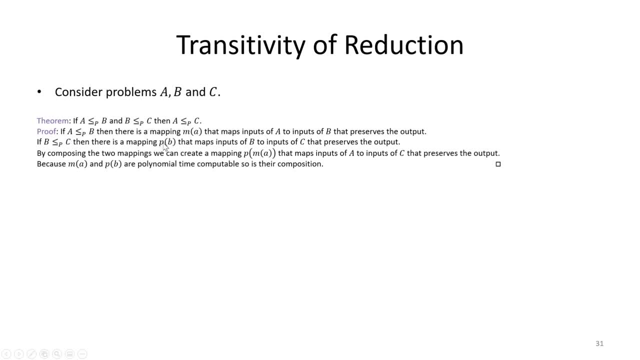 to c, then the same thing is true here, except I'm going to change it up. I'm going to call it p instead of n, and it takes inputs to b and maps them to inputs to c and again preserves the outputs. yeses to yes, nos to nos- Again. polynomial time computing too, Then, what we're going to do? 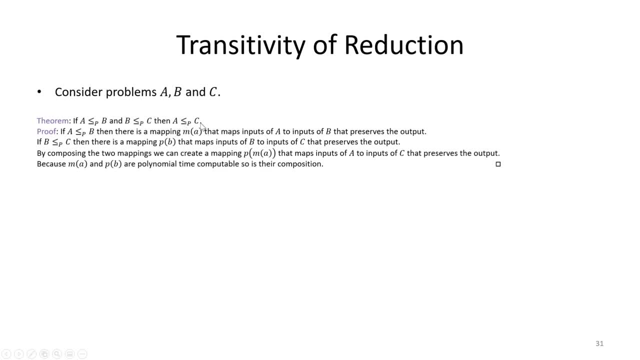 say, we want to map a's to c's. now I'm just going to take my mapping that takes a's and spits out b's and then put that inside my mapping that takes b's and spits out c's. So I'll plug into this. 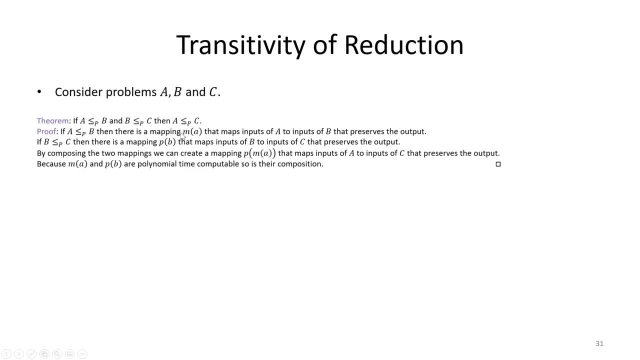 composed mapping in a and what will come out is a- c. That's what I want Again. since m maps yeses to yeses and p maps yeses to yeses, and same thing for nos. our new composed mapping must also preserve the output. The only last thing we need to confirm is that 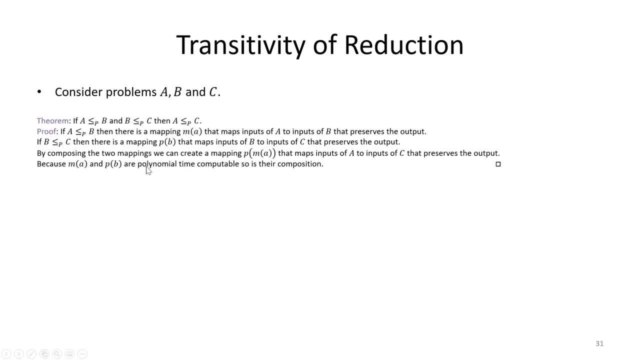 computing both mappings is a polynomial plus a polynomial, so we still have polynomial computation. So this is the idea that Karp applied. Here's again. so everything on the left here this is the work of Cook and Levin, Taking all the NP problems and showing they reduce to sat. Karp takes sat and reduces it to his favorite. 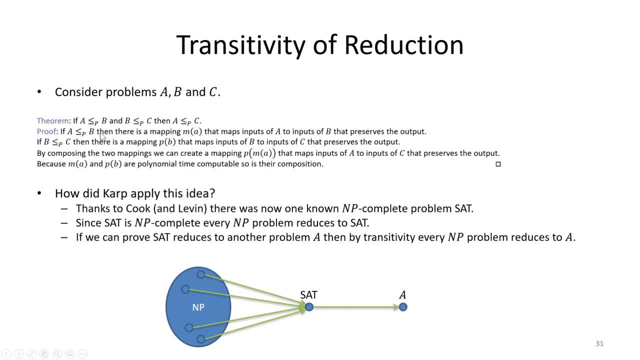 problem a and then through transitivity, through this theorem here, we get that, since, say, a reduces to b and b reduces to c, we get the a reduces to c, the link that we want. All of the problems in NP must then reduce to a. So Cook and Levin did infinite proofs all at once. 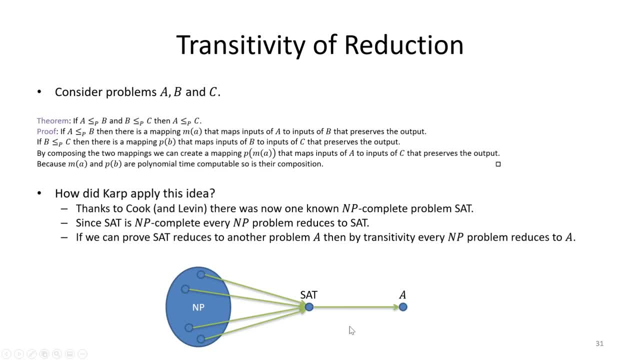 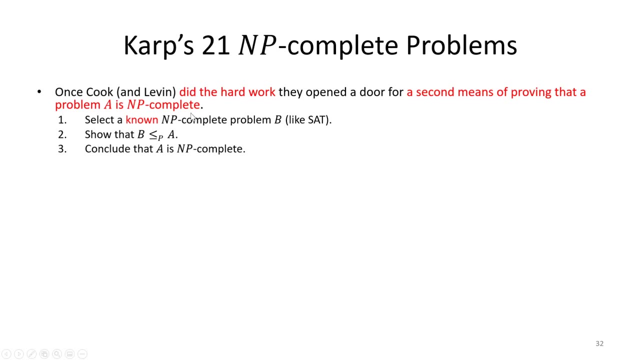 But we only have to do one reduction, Infinite reductions at once. we only have to do one reduction if we want to prove other theorems. are NP complete as well? So this is our new strategy. I think I just said it on the previous slide, but let's look at it sort of. 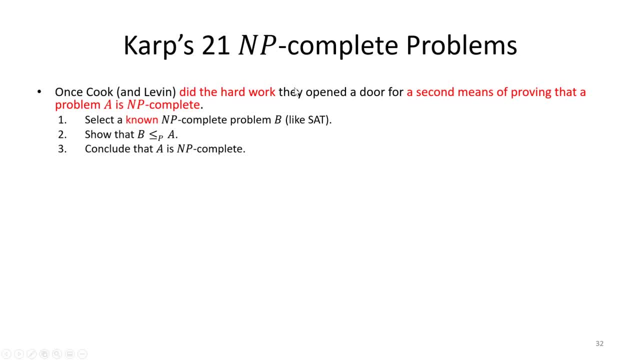 verbalized here. If you want to show some problem is NP complete- Say you've got some problem a that you want to show is NP complete- First thing you need is some other problem that you already know is NP complete. This process won't get started properly unless we already 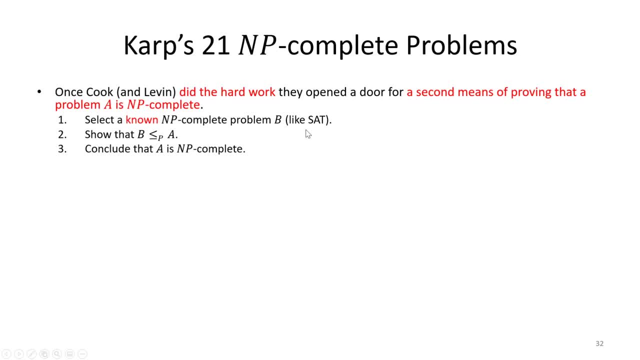 have one problem we already know is NP complete. So again, this is why SAT plays an important role. Now we need to do a reduction. Now here's the important thing we need to take the one we know is it is NP complete B and reduce it to the one. 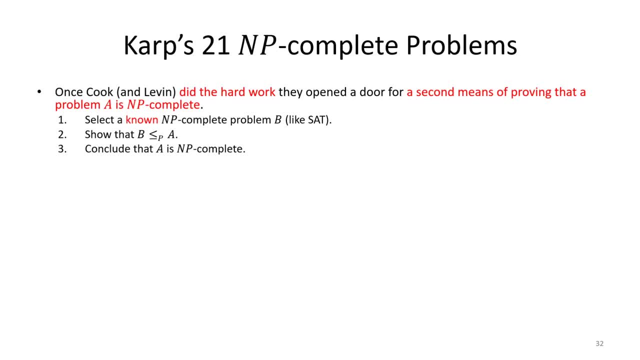 we don't know, is NP complete? and this is is, for many, many people, very counterintuitive. Usually, when we reduce problems, we want to take the one we don't know anything about and reduce it to the one we do know something about. That's what our idea of solving a problem using the solution from another. 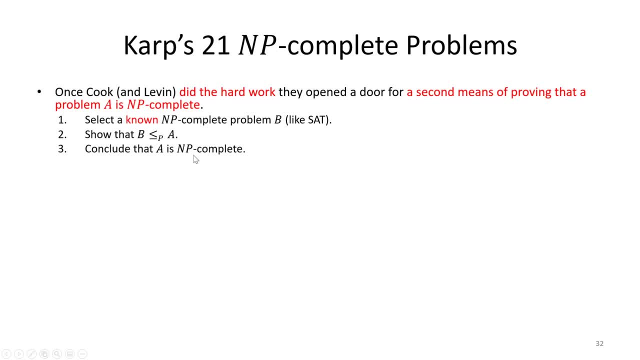 one. But here we got to put them in reverse order to prove NP completeness. That is, take the one we know is NP complete and reduce it to A. And the reason is again this no harder relationship. We're trying to show that that B, the NP complete problem, is no harder than the problem A meaning A. 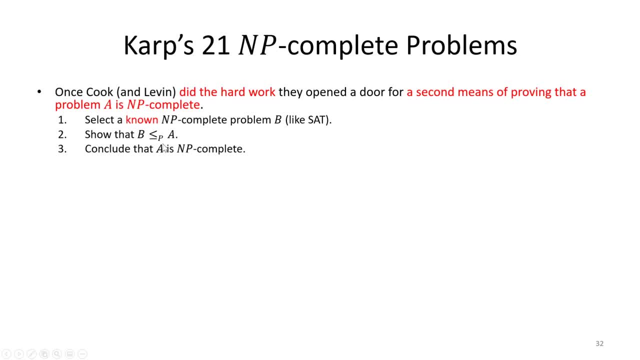 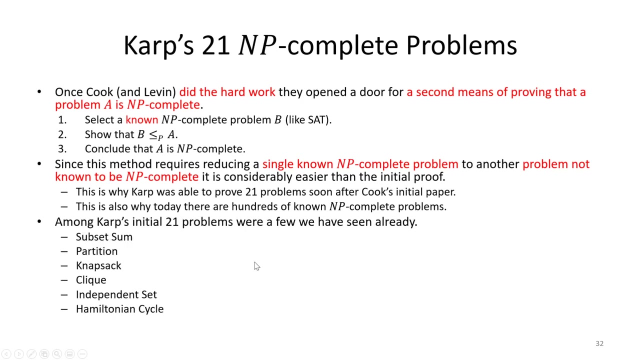 might be harder than it. Okay, and that's what we're trying to establish here. Okay, finally, if we show that reduction, we simply conclude that A is NP complete as well. So, again, Karp was able to use this to come up with 21 new problems, and among: 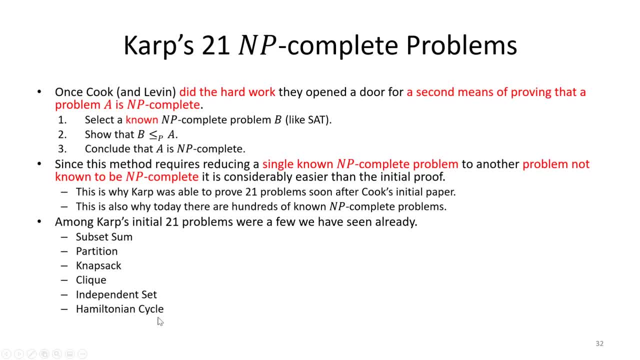 Karp's initial problems were at least versions of some of these problems. They weren't exactly the same problems as we've seen them, but subset sum, partition, knapsack, clique, independent set and Hamiltonian cycle all appeared in one version or another on his list of 21 problems. 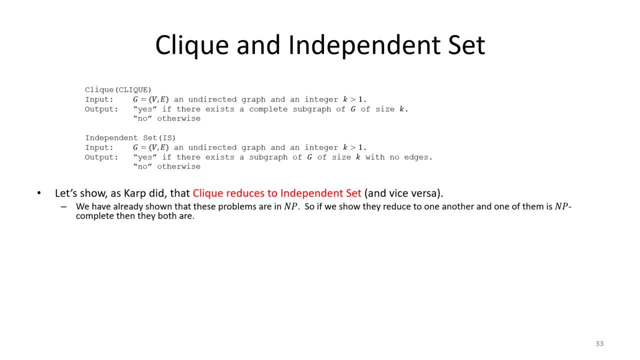 So I do want to sort of finish this video here with our first reduction, and because some of these reductions become very involved in several pages, as I mentioned in Gary and Johnson, similarly for Karp's initial reductions, many of them can be quite involved. I want to start with some fairly fairly simple. 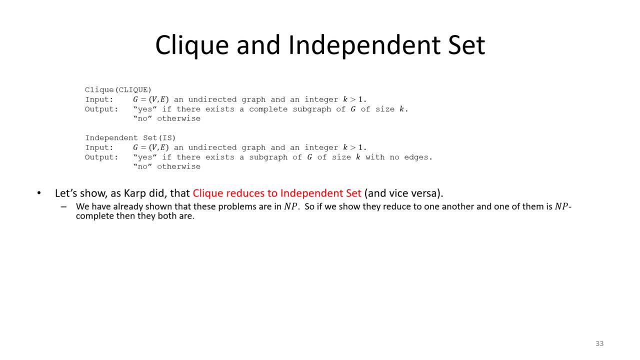 ones, And so the simplest one I want to start out with here involves clique and independent set. Let's just quickly remind ourselves what these two problems are and the decision made. So we're going to look at a problem version of them: Clique and independent set. here are 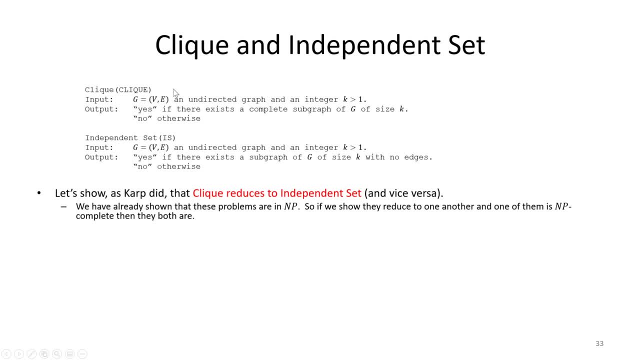 problems. they're graph problems. You're going to take as input an undirected graph and some threshold that helps it make it in a decision problem here: K some threshold And we're going to ask something about a subgraph. Now, clique is. 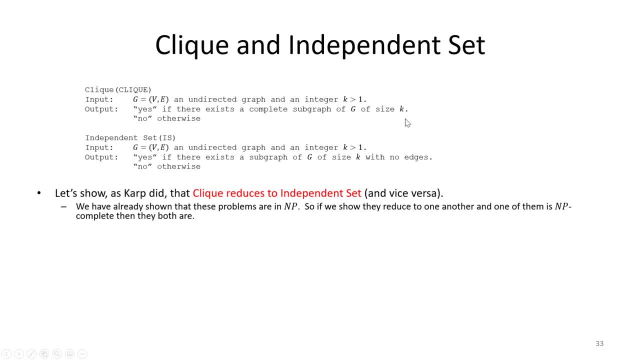 asking: can you find a complete subgraph of size K, Remember that's one where all the edges exist, And then independent set is sort of asking an opposite question. can you find a subgraph with no edges in it at all? Okay, again of the appropriate. 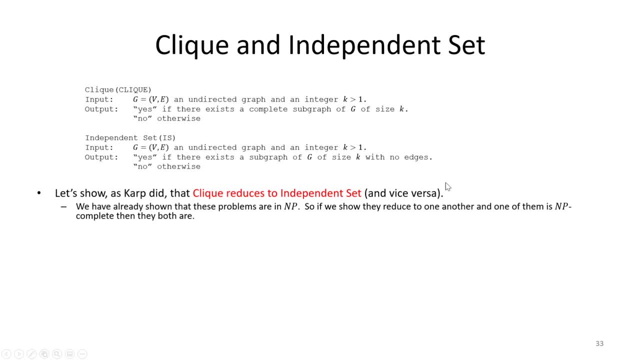 size K. So we want to show how these two problems are closely related. We already see there's sort of a similarity in their definition, but we want to use a reduction to prove that. Okay, so let's say we're going to build a mapping. now To build the mapping we need. 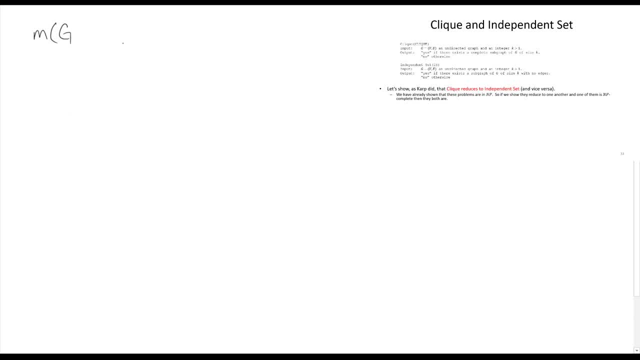 to use the input that's coming in. So remember, we're mapping from one input to another. So here I'm going to assume here for the moment: let's say we're doing clique reduces to independent set and, and that way we know which direction we're going here. so the input to clique is just this, input g and maybe 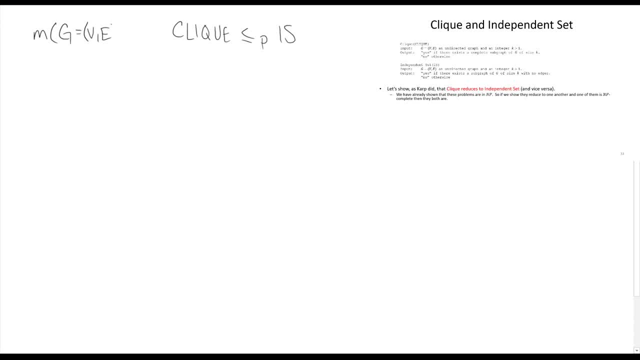 I'll just be clear here: equals v, e and then a k. remember there's this integer k. and then sometimes the way I like to do this is I might just go down here and say: well, what this mapping is supposed to do is return something else, an input to something else. well, what input to independent set? now, if I'm 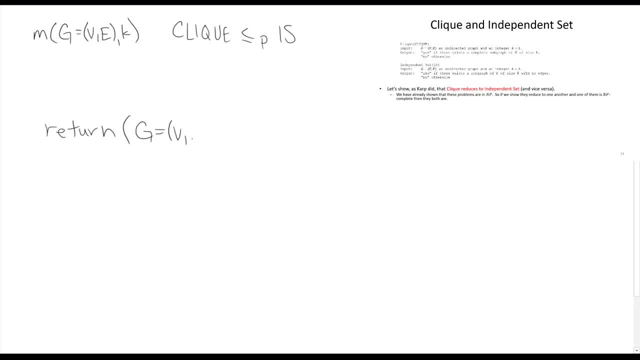 a little sloppy. I might say: well, that's a g equals a v, and an e and a k, and if I just write it like this, that implies I'm taking exactly the value from above and plugging it in below. now, some reductions might work that way, but that's not usually a very good reduction because this: 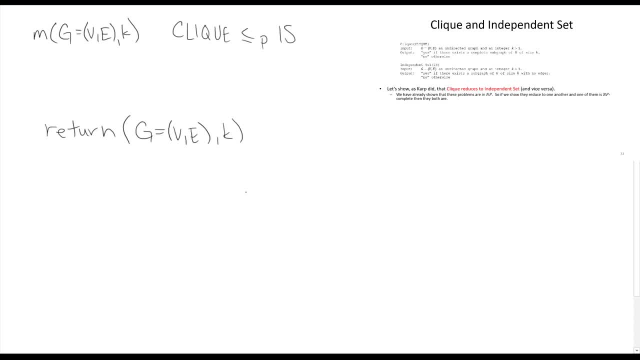 reduction is not going to preserve our output. remember, that's the key thing we want. if this input here- this was an input to clique, if it has a clique of size k, a complete subgraph of size k, then we want this graph down here to have an independent set of size k and we can't establish that by just handing the same. 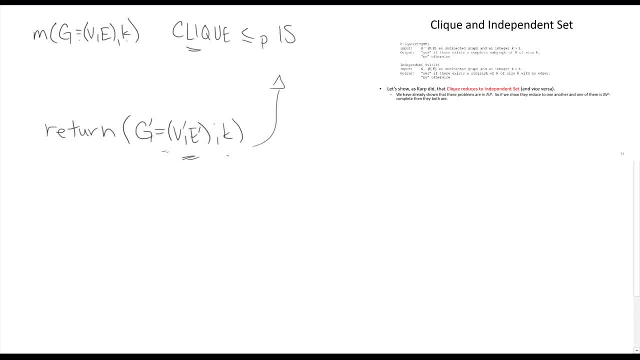 graph over. so, to get myself warmed up, I'm going to say: let's, let's do this. let's change the name here to g prime, v prime, e prime and k prime, keeping in mind that these might be different. they might not be different. okay, now to do this. 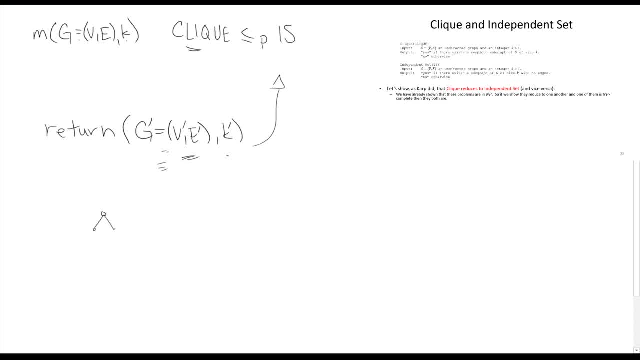 what I want to do is: I want to look at a graph here. I don't know what I'm making. here is sort of I wanted to make a clique in there, so there, I made a clique. okay, so imagine this was our input, graph G, and our K here was: let's see one, two, three, four, five, six, seven, seven, eight, and now we have a. 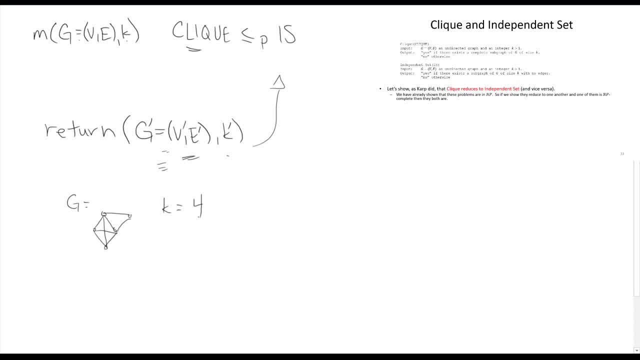 there's four vertices in that clique, so let's say it's four. or there's another possibility: let's say it's five. why? because if it's four we should say yes, if it's five we should say no. right now, what we want to do through our process. 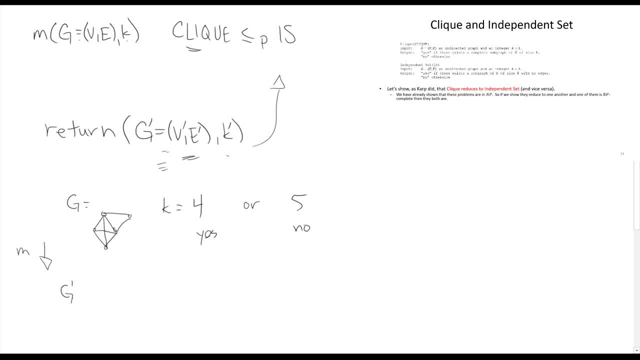 here M is. we want to come up with a G prime and a K prime. K prime- okay. how can we do that? now, if we just look at this graph here, we'll notice that the fact that there's a clique in here doesn't imply anything about the size of the. 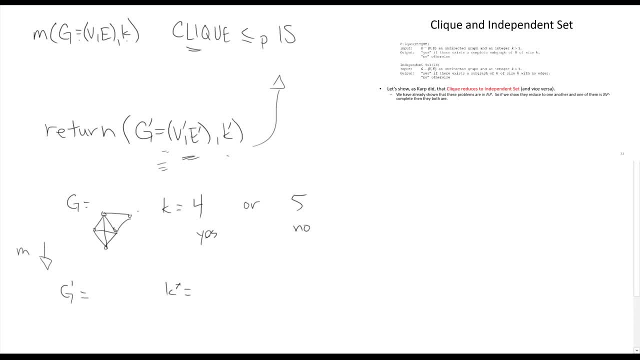 largest independent set in here. maybe it's do. it looks like okay, that's not going to help us unless we inspect the graph. we don't want to inspect the graph, but what we can realize here is that if we have a clique in here, a size for that. 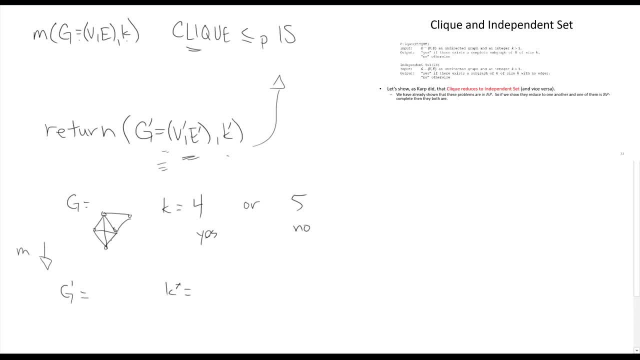 if we took out all those edges. so follow me for a second. that would create a second 거 I can do, if what I do isегere this clean omega x that is lighter than that. if we're doing 커어� receptor, and I'm doing, 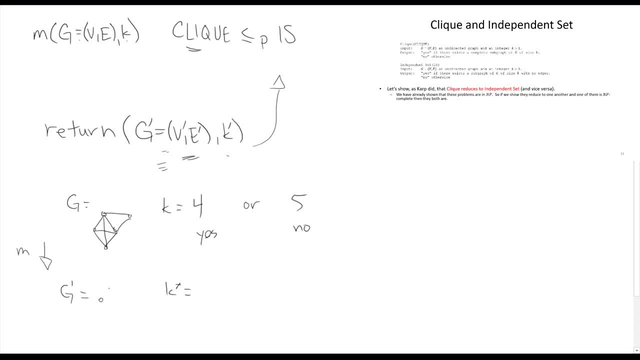 that and once we get a class over what would that work? this equation perhaps create an independent set of size four. So one step we could do here is we could say: well, delete all the edges. Now I need to be careful here. We don't want to say delete all the edges. 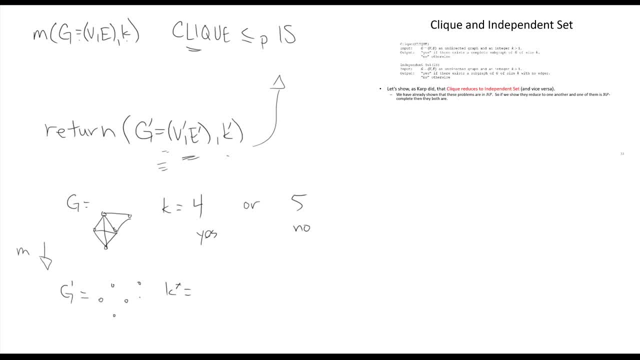 in the clique. That's certainly something I could write up here, But if I did, I'm no longer going to be polynomial time computable, because that implies I can find the clique. If I can find the clique in polynomial time, well then you're smarter than I am. I don't know how to do that. 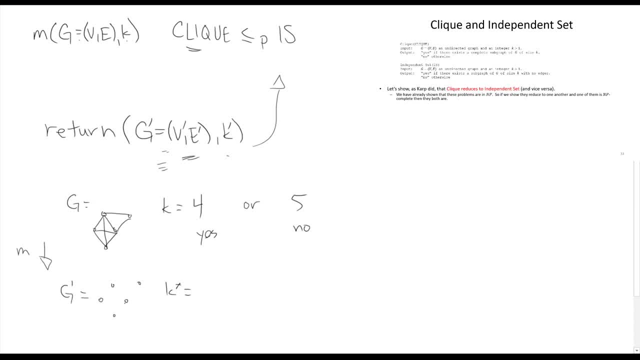 So what we want to do here- and we don't want to delete all the vertices, because you'll notice- here, let's say we did k, prime equals four. here This part would work. This is a. yes, This has a clique of size four After deleting all the edges. yes, I have an independent set of size four In. 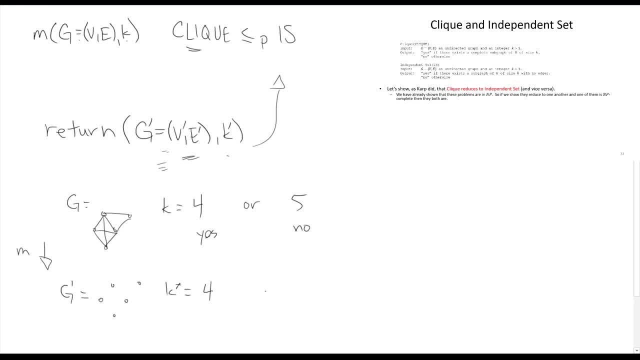 fact, I have an independent set of size. five now, Okay, And that's why, if I put in five as my input, the problem with this graph over here is I would still say yes on it And I should Right. This should be a no. That's what it says up here. So I took out all the edges that were in. 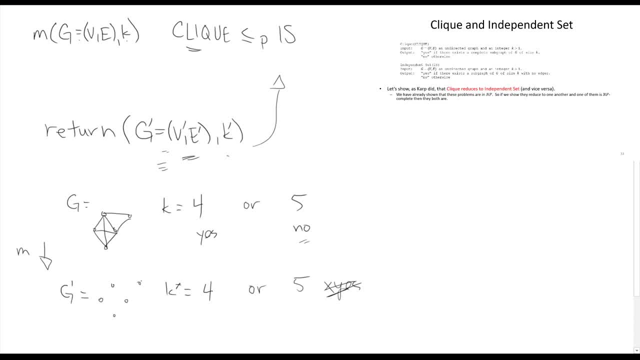 the original graph. What I need to do is I need to put in edges that were not in the original graph, So this vertex was not connected to these two. It was only connected to these two By adding in the edges that were not in the original graph. now, I would say no on this one, which is right, And I. 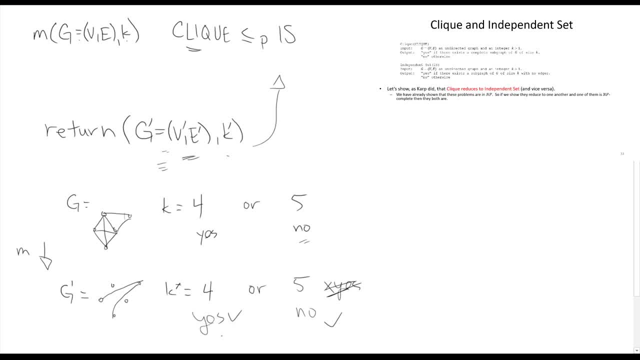 would say yes on this one, And I would say yes on this one, And I would say no on this one, And I would say yes on this one And I would say yes on this one, which also seems like it's right. So, in order. 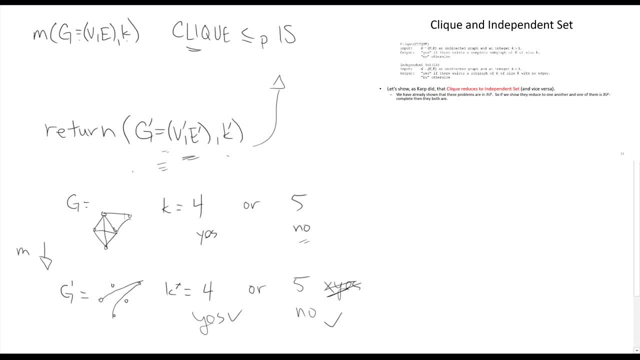 to do this, we now need to finish our mapping here. So how do we describe this? What is this? This is what we might call the complement graph. Okay, In the complement graph, all of the vertices are the same as the original graph, So v prime is the same, But our edge set is going to be the complement edge. 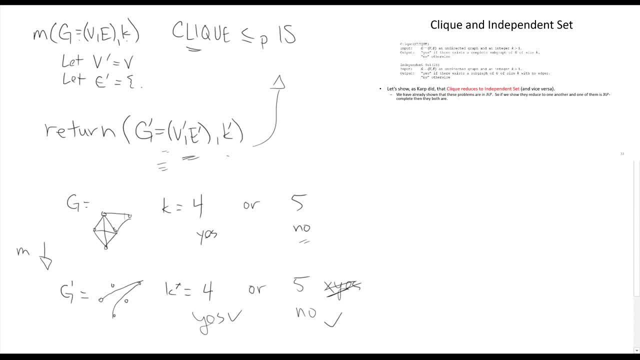 set. so I'm going to say it's all of the edges that are not in the original edge set. and then we saw that we didn't need to change our k. our k was fine, so I'll let k prime be equal to k. so this here is our mapping m. 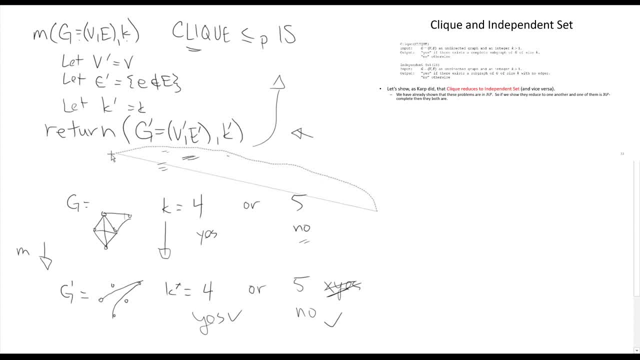 that mapped inputs from clique into inputs to independent set. so now what I want to do is argue that this is correct, that we haven't messed it up, and to do that we're going to do another kind of structure that I've shown in the previous videos. 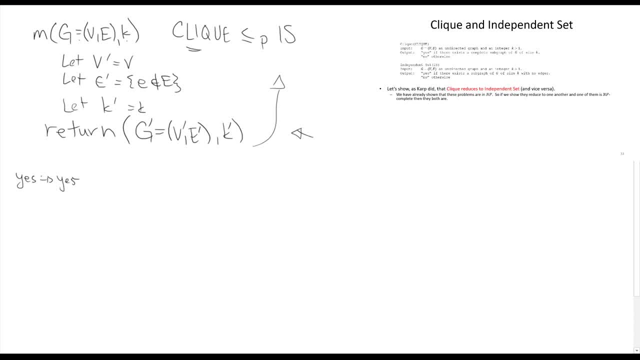 which is a yes implies yes. we're still going to have to prove a yes if and only if here. okay, but it's a different kind now. now, what we're trying to show is that we preserve the output meaning yes to clique. so this one is yes to clique. 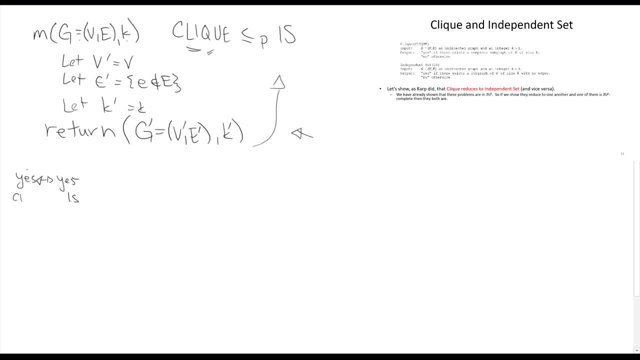 it means yes to independent set. and then back again. now I usually like to prove this as to yes implies yes. so let's do our first direction here, where we're going to do: yes to clique implies yes to independent set. so I'm going to assume that g has a complete subgraph of size k. 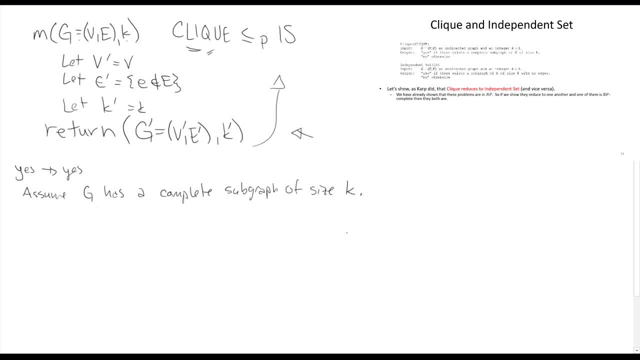 now remember. that's exactly how we start off some of our proofs here in the previous bit for verifiers. we're starting out the same way, because we're assuming this is a yes instance. okay, so we assume we should say yes on it. okay, but what are we trying to argue is now different. 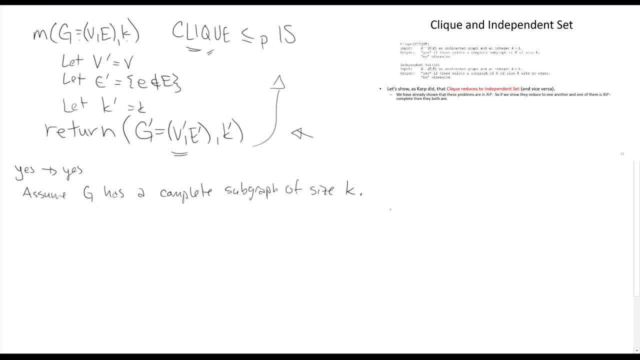 we want to argue that the thing that we map to at the end is also a yes instance. okay, so every edge in this clique that this complete subgraph does not exist in g prime because of this transformation here. so what does that mean? so that means g prime must have a independent. 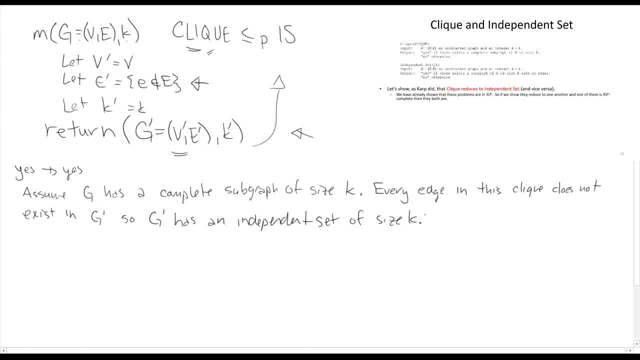 set of size of size k, and that was what we were trying to prove. we were trying to prove that g prime was a yes instance of independent set. okay, so that was the yes implies yes. now we could do no implies no, that would be assume. this is no, therefore no. 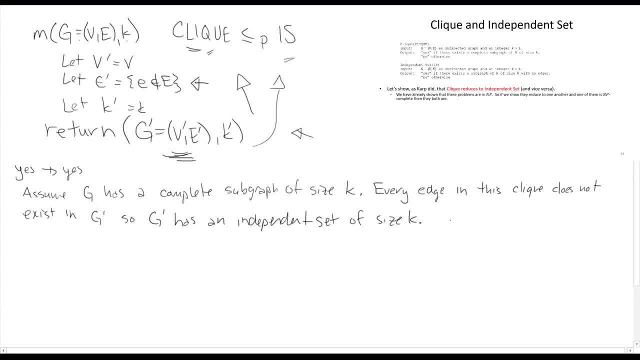 but I actually like to reason backwards, because if we do it right, we follow the exact same reasoning we did here, but just backwards, and if you get a little practice on this, you start being able to phrase your proofs properly. so you can do the whole if and only if, all in one tackle. 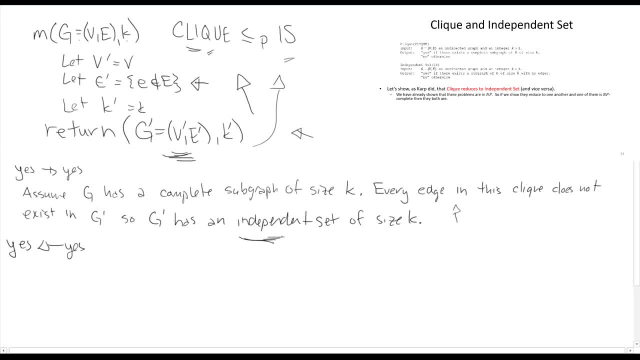 so let's go backwards. going backwards means just starting where we ended before and ending where we started before. so we're going to start by saying: assume g prime has the independent set of size k, and we're trying to argue then that the original graph must have had a clique of size k. 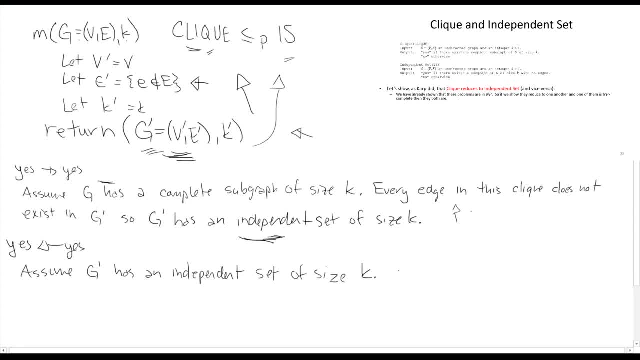 so we're going to use the same idea here, that is, every- let's call it- missing edge here. so every missing edge in this independent set exists in g, so g has a clique of size k. we can see the argument here flows almost exactly the same backwards. 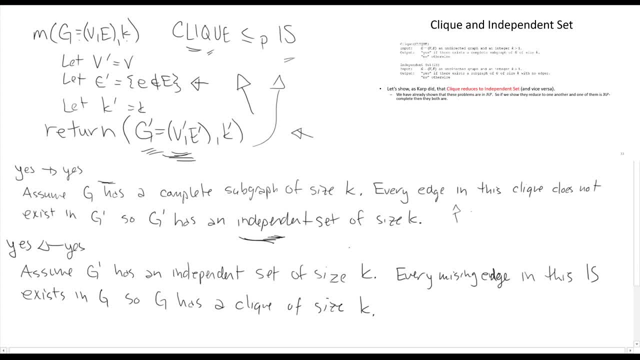 as it did forwards, using the same logic and reasoning, and so that's one reason why I like to do yes implies yes backwards. now, the other thing I would comment about this reduction is: this is the simplest reduction that you're going to encounter, because clique and independent set are very closely related. 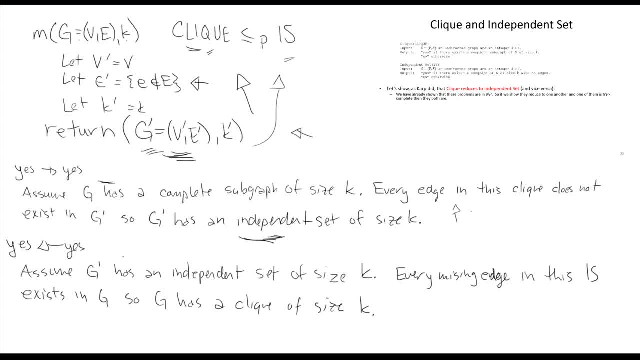 they're not. they're not exactly complement problems, but they have. because of the complement graph figuring in here, they almost have that complementary nature. now, not all problems are going to have that very simple, close relationship, but when you're coming up with reductions you always want to select a problem. 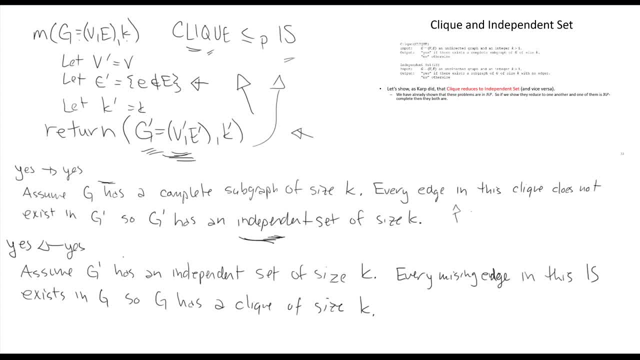 that seems close by. okay. so if you've got a graph problem, you might want to pick another graph problem. if you've got a set of integers problem, you might want to pick a set of integers problem, and so on. it becomes harder to move between domains. okay, but that doesn't mean it's impossible. 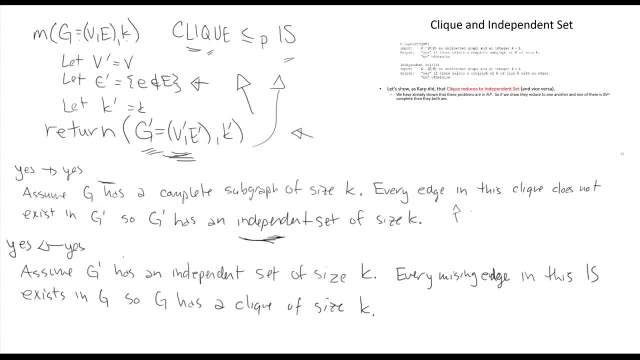 and then certainly many of the interesting proofs that Karp provided are of that nature. now, if you're interested, please do take a look at some of Karp's proofs, or Gary and Johnson's proofs as well, but in my final couple videos in this series I am going to just review a few more.